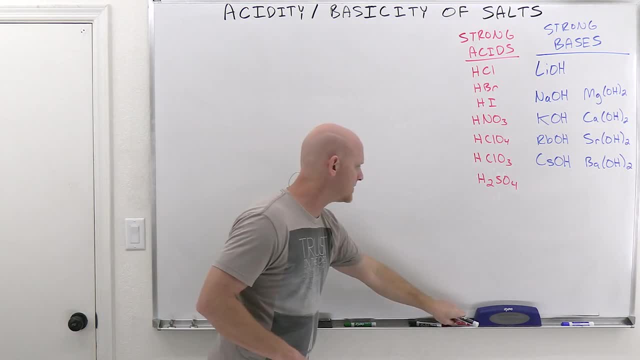 remember. So the big thing we should look at here is: we're going to take a look at cations and we're going to look at anions and treat them separately and go from there. And what you should realize is that if we look at the Lewis definition for 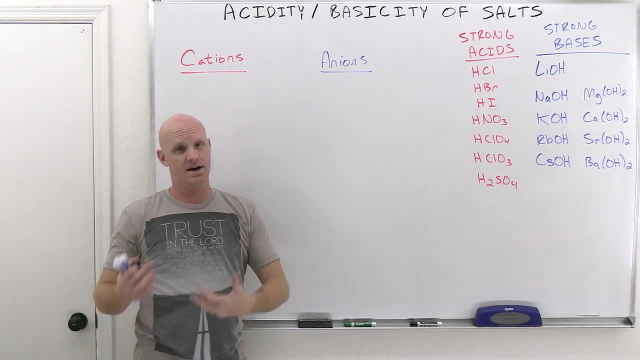 acids and bases. it'll kind of give us an idea of whether we should expect cations and anions to be acids or bases. So a Lewis acid is an electron acceptor, and if I was looking at cations or anions and saying which one's more likely to accept, 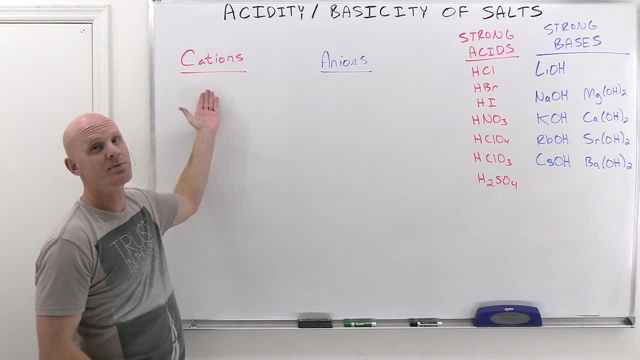 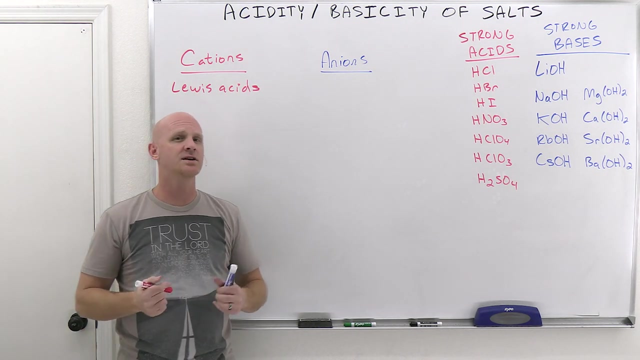 electrons. Well, electrons are negative. It's the cations that are positive, and so you'd expect cations to be electron acceptors, and so cations are usually Lewis acids. We talked about this back in the first lesson in the chapter. We talked about acids that might qualify under Lewis's. 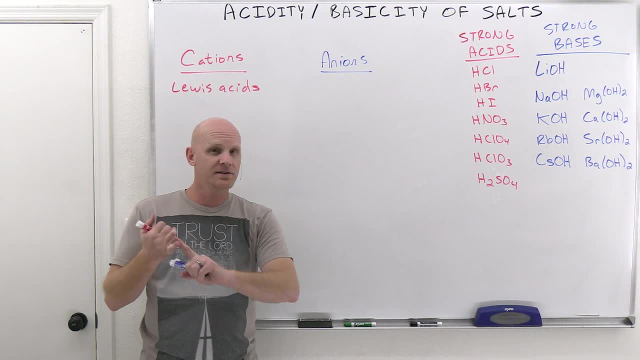 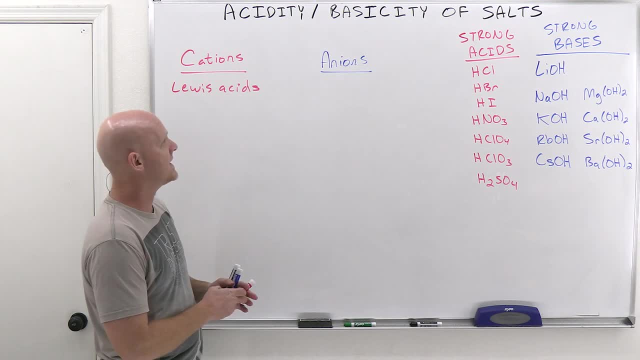 compounds which have an empty orbital, and then boron-containing compounds. So we talked about metal ions, metal cations. Now, on the other hand, anions having a negative charge, they are much more likely to be electron pair donors. so, Lewis, 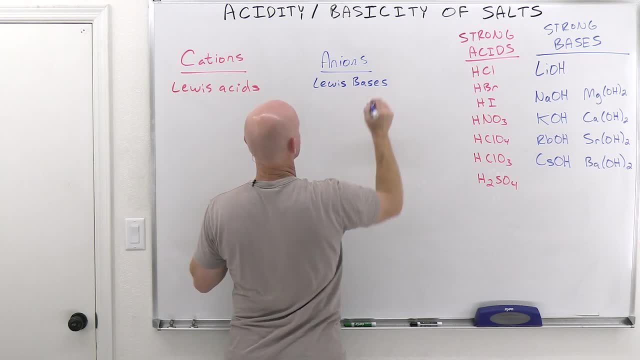 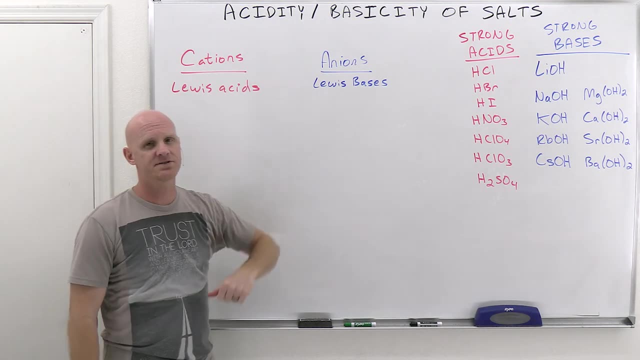 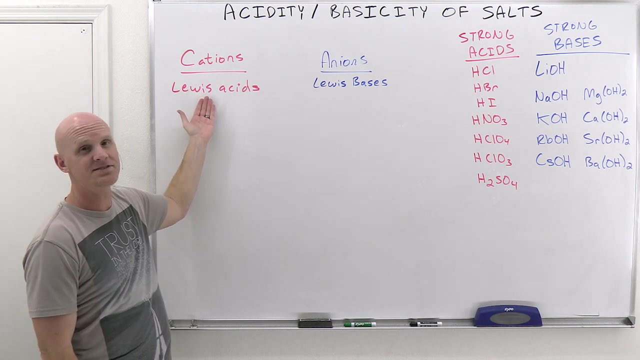 bases, or in many cases Bronsted bases, or even Arrhenius bases as well. So we're going to kind of look at just the Lewis definitions for this, because it's easy to associate them with cations and anions. Cations might be great. electron acceptor, I'm sorry, yes, electron acceptors. 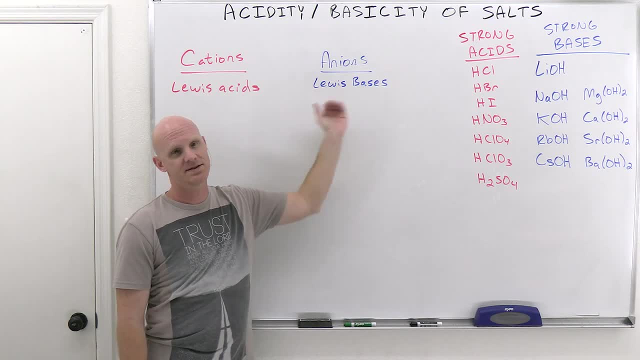 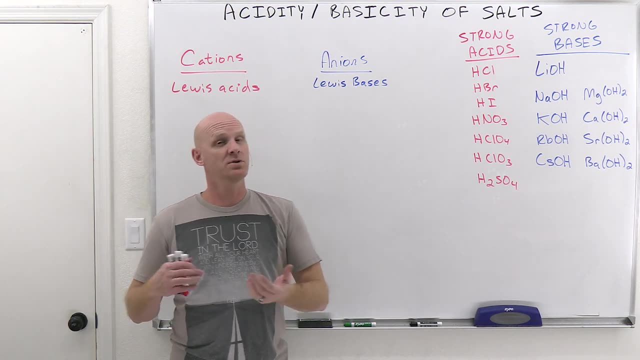 Lewis acids and these might be great electron donors- Lewis bases. And so when you see a cation, you should think, good chance it's an acid. When you see an anion, it's a good chance it's a base, because most cations are acidic and most anions 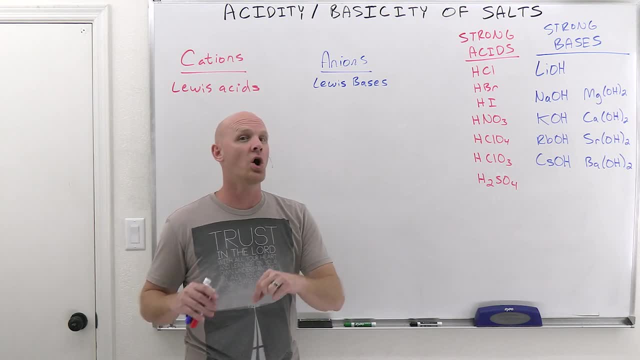 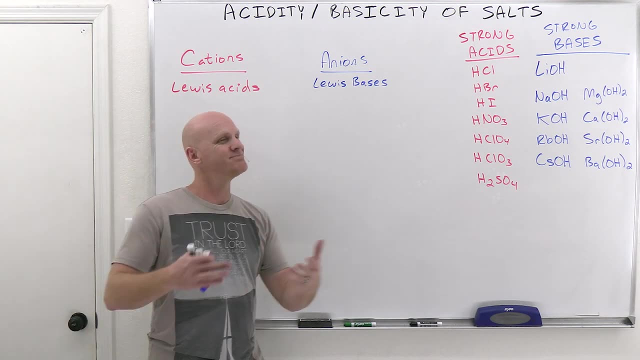 are basic And the key is you're going to remember which ones aren't, because there's only a few cations that are not acidic and there's only a few anions that are not basic. As long as you remember which ones aren't, then you'll know that all the rest are either acidic for cations or basic for. 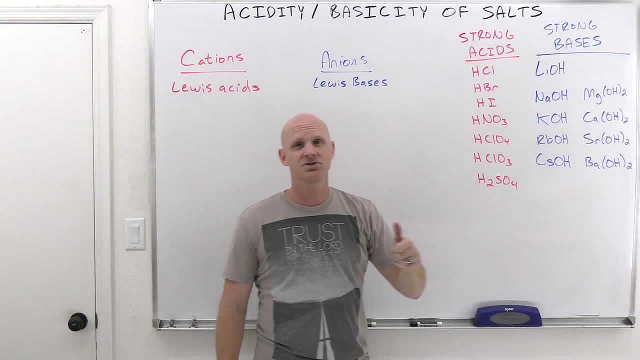 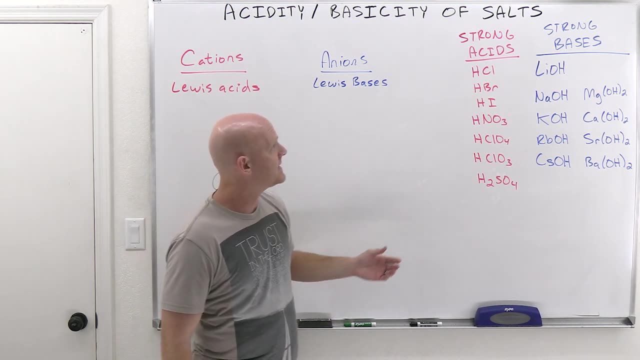 anions And knowing your strong acids or bases. that is your key to remembering which ones are not acidic and not basic. So we're actually going to start with the anions here. So if you take a look at your strong acids- so we've emphasized this a couple of times throughout the chapter. 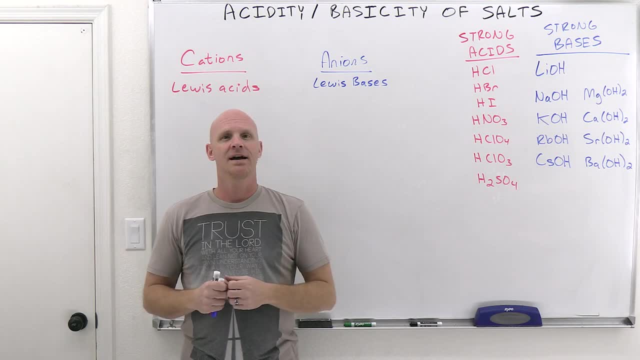 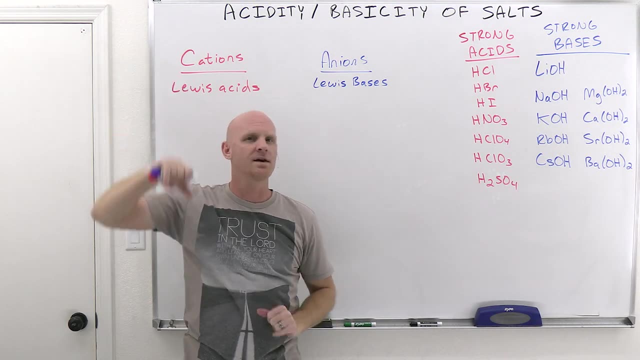 that the stronger an acid, the weaker the conjugate base. And so it turns out. you know, if you've got a strong acid at the top of the list, its conjugate base is so weak that it has zero ability to act as a base in water. I'm going to call it a negligible. 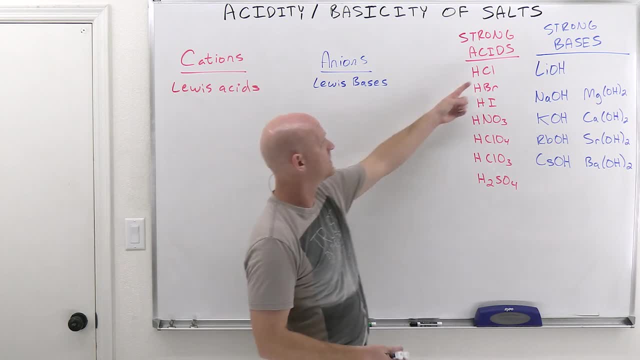 Base. So and so in this case, if you take a look at chloride bromide, iodide nitrate, perchlorate and chlorate- and we'll talk about him, special uh bisulfate in here in a little. 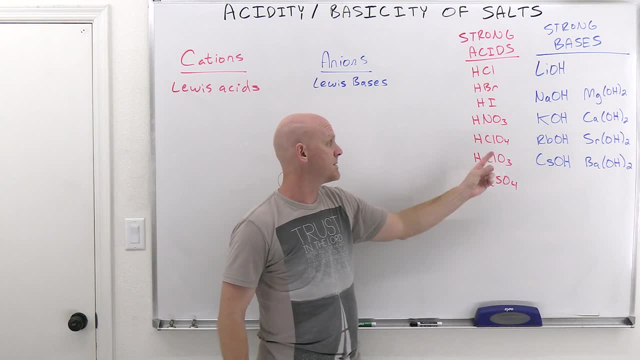 bit So, but the first six: chloride bromide, iodide nitrate, chlorate- I'm sorry, perchlorate and chlorate. So it turns out they are such weak conjugate bases that they have no ability to act. 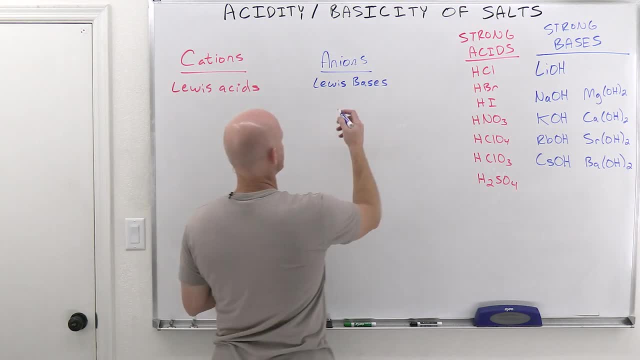 as a base in water. They are negligible bases, And so I'm going to put those special here. We're going to talk about chloride, bromide, iodide nitrate, perchlorate and chlorate, And these are the ones that we are going to call. 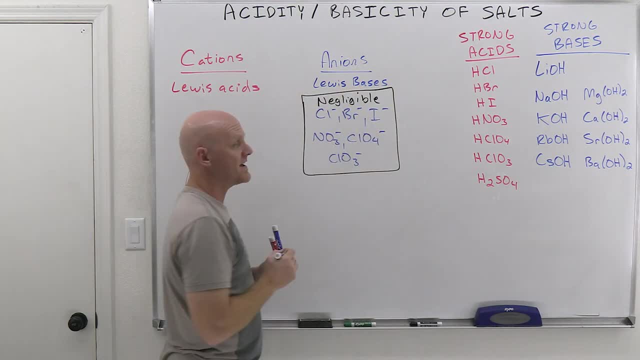 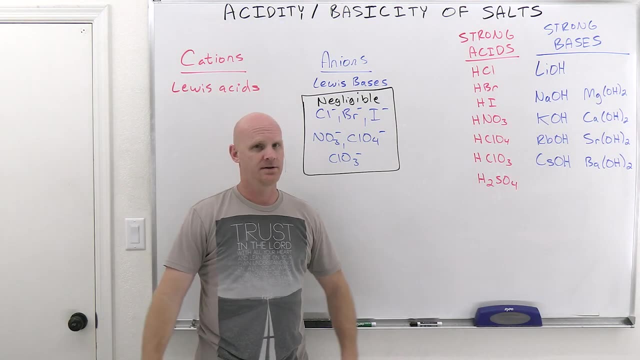 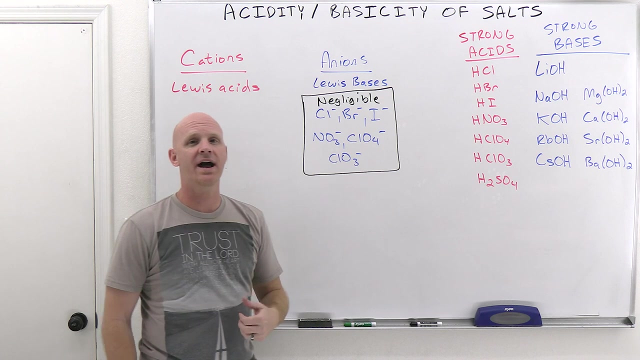 negligible. They are your negligible conjugate bases. They don't affect the pH of water at all. So again, when you see an anion, you should think it's probably a base. Just not these guys. They're conjugate bases of six out of the seven strong acids. and they're such weak conjugate bases. 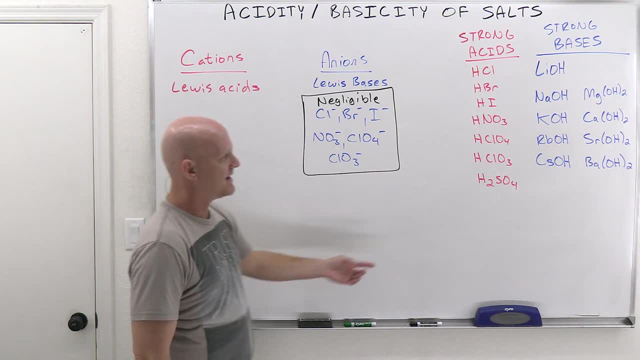 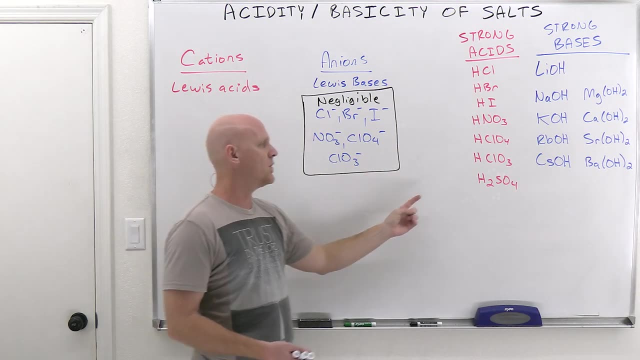 that they're not going to act as a base in water. Okay now, H2SO4 is a little bit special here. So H2SO4 is the only one of these that's polyprotic, and you might recall that only the first H. 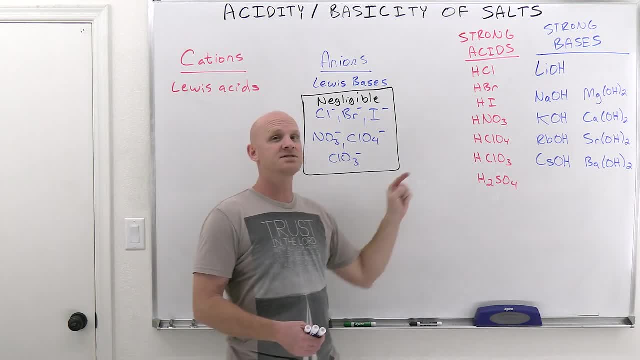 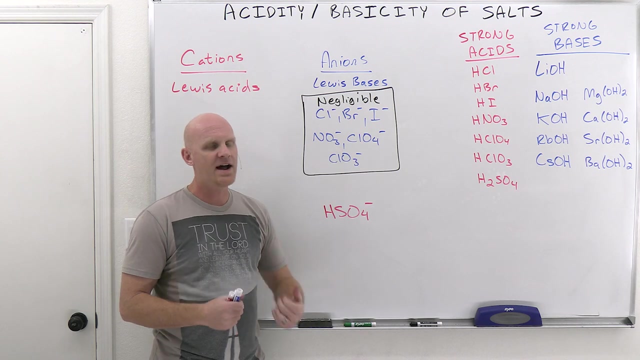 dissociates 100%, the second one only partially. The first H is a strong acid, the second one's only a weak acid. Well, once he donates one H, he's going to look like HSO4- and we just said he's a weak acid. So that's an exception of all exceptions, right? So 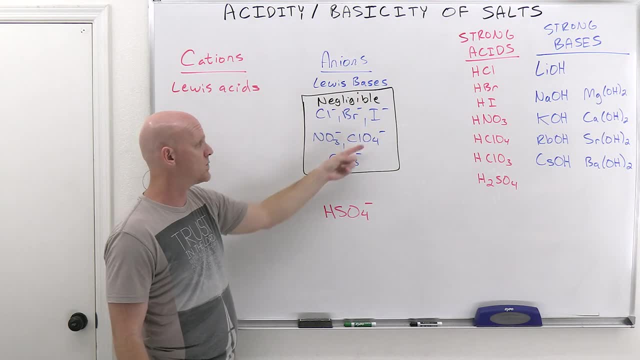 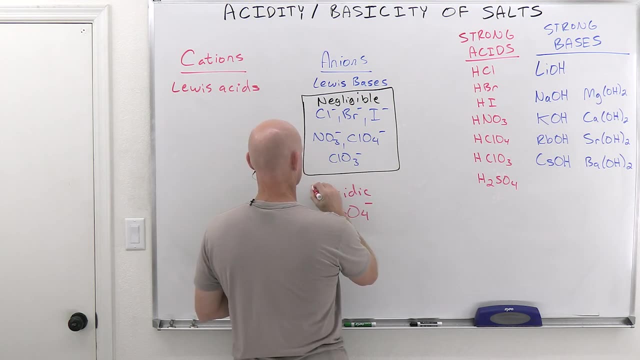 he's an anion. Almost all anions are bases. Here's the ones that are neutral, but here's one that actually is acidic, And he's not the only one, but probably the only one you're likely to encounter. So there's a couple of them. 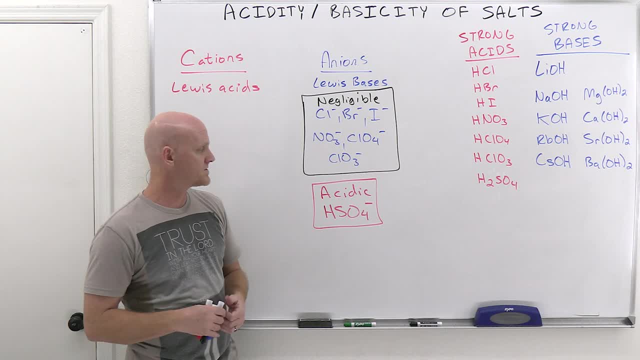 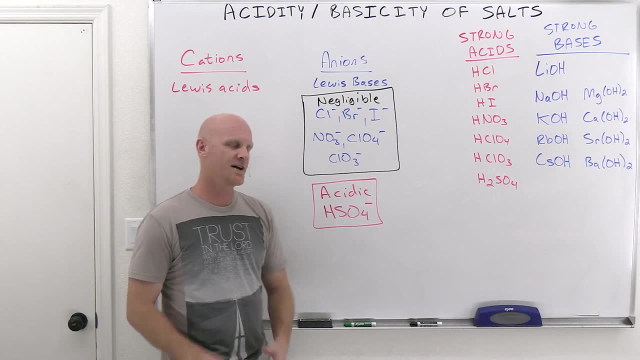 A couple. one of note: like turns out, oxalic acid's also a diprotic acid, and the monoprotic version is also acidic, but you're not likely to encounter that. So this is the most likely one you're going to encounter, And so the way you should treat anions then is you should know that. 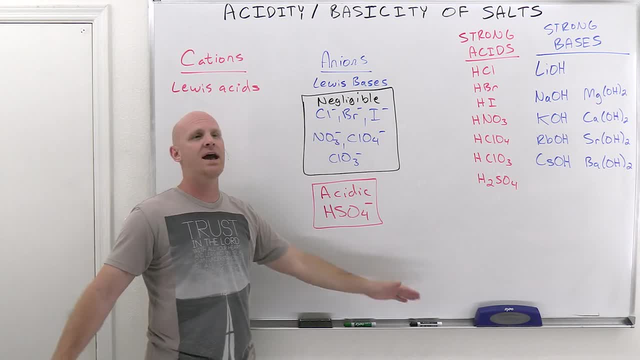 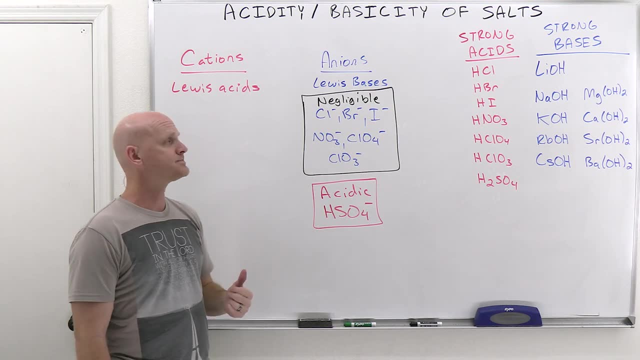 these are the neutral ones. there's one acidic one, and any other anion outside of these is going to be a base, so an electron donor. That's the way it works. Now, cation's on the other side, So it. 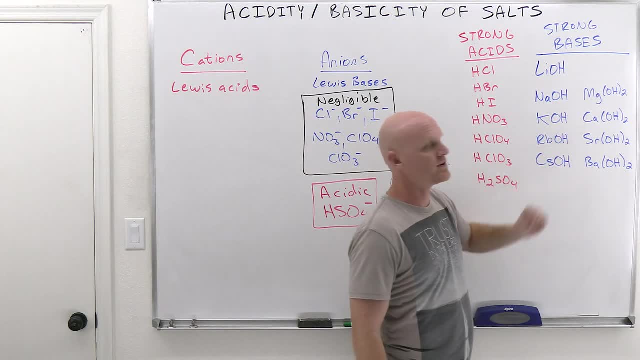 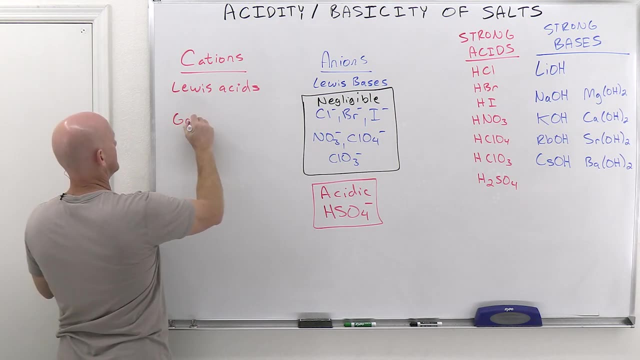 turns out that the group one metal ions and the group two metal ions, those are going to be your negligible ones over here, And so in this case I'm just going to put group one metals, group two metals. these are now the negligible ones. 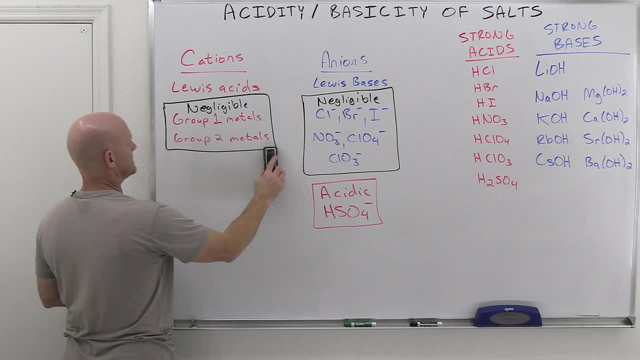 So, but it turns out they're not alone. So we're gonna make a little room, I guess, in this box and put transition metals that are only plus one. So I'm going to call it a transition metal with just a plus one charge. We'll add them in here as well. 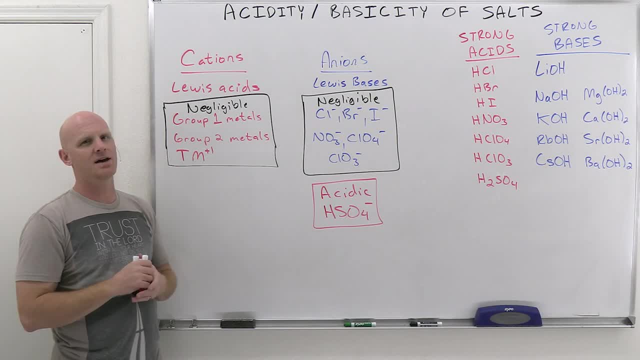 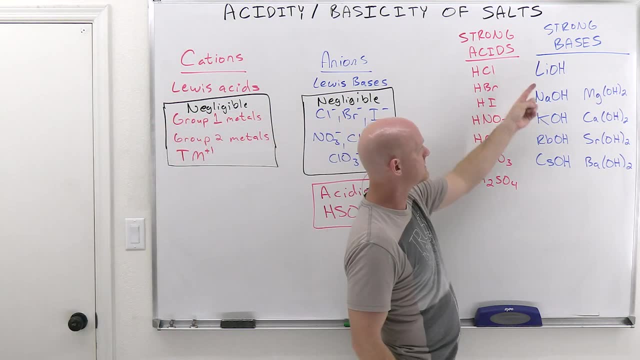 Technically. there's some other oddball ones under the staircase on the periodic table that are even when they're plus two, but you're just not likely to encounter this. So I'm going to sum it up like this: So, group one: metals like lithium, sodium, potassium, rubidium, cesium, and then the group two, metals like 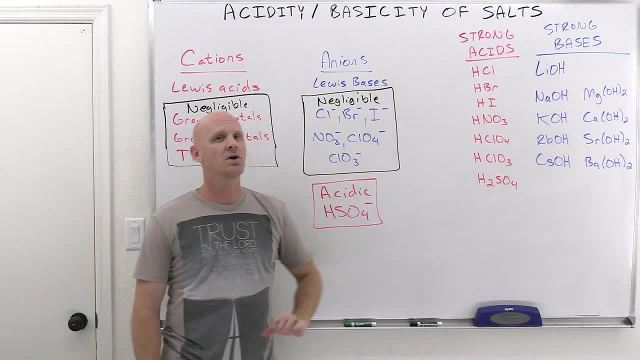 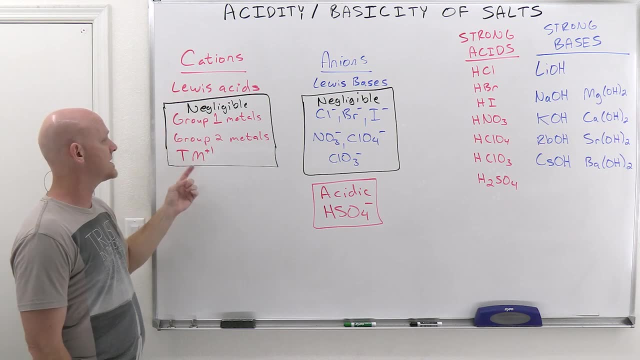 magnesium, calcium, strontium, barium. when you encounter them in a salt they are negligible. But pretty much any other cation you're likely to see outside of the group one, the group twos, and if a transition metal is only plus one, they're going to be negligible as well. 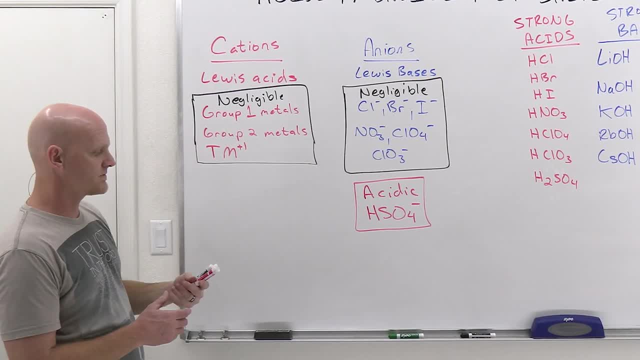 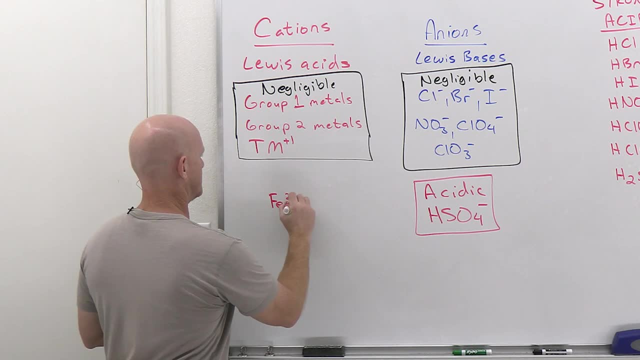 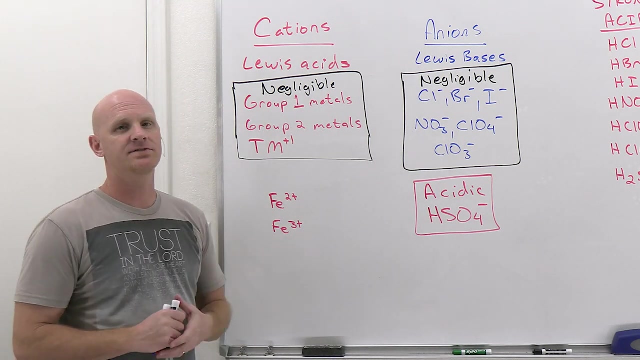 And one thing you should realize about this: there's a couple of trends involving these Lewis acids for metal ions. So if you were to compare, say like Fe2+ and Fe3+, and just your gut, which one of these is more likely to act as a stronger Lewis? 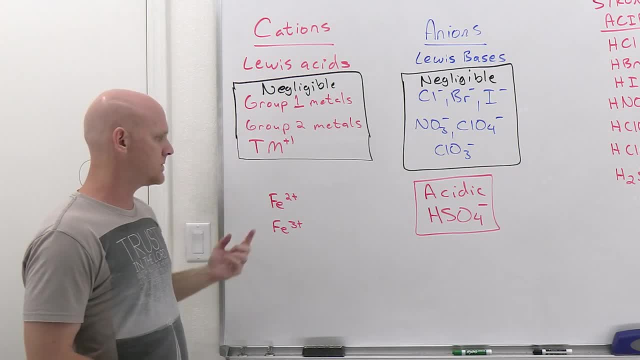 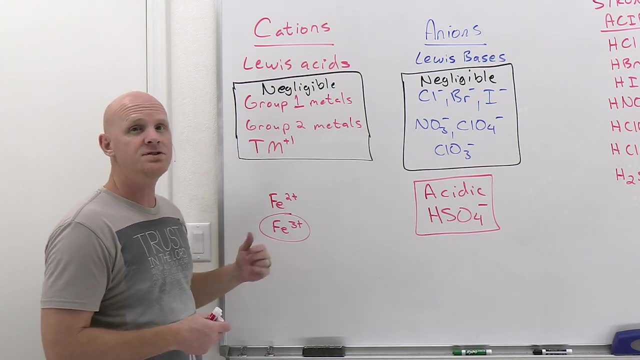 acid, a stronger electron pair acceptor, Well, the one that's more positive, for sure, And that is definitely the way it is. So if you've got two of the same metal but different charges, it turns out the more positively charged they are, the stronger. 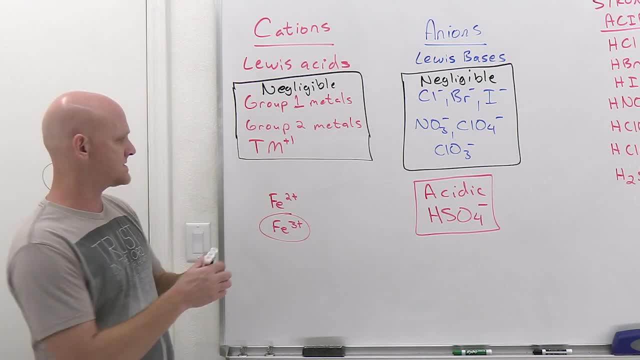 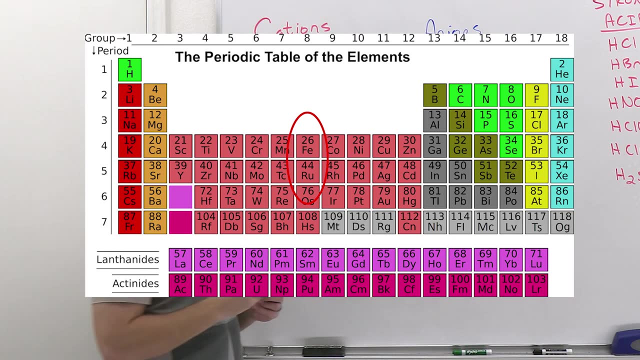 the acid. Now, the other comparison you're going to want to be aware of is based on size. So if I have Fe2+ and Ruthenium 2+, so it turns out a smaller one can bring those electrons closer to its nucleus because it just got a smaller size. 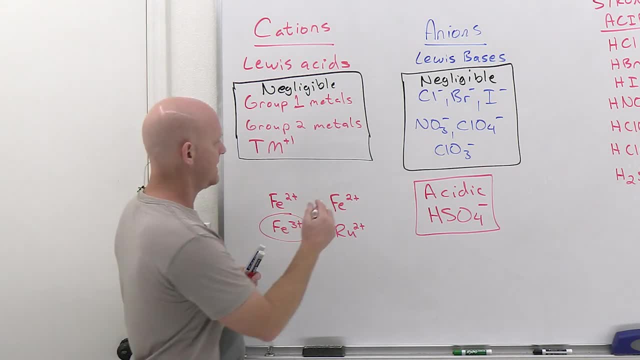 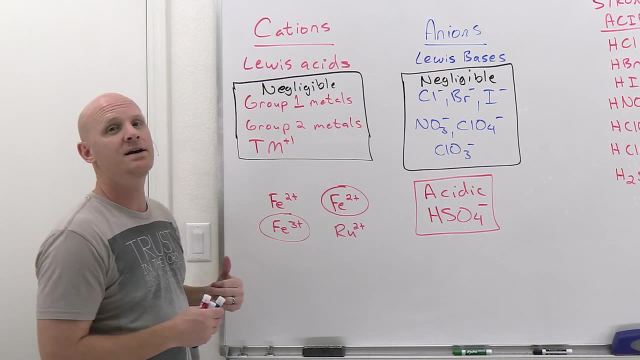 and that's going to make it a better electron acceptor as well, And so in this case Fe2+ is better than Ruthenium 2+ right below it on the periodic table, So both charge can play a role in how strong the Lewis acid is, but size can play a role as well. 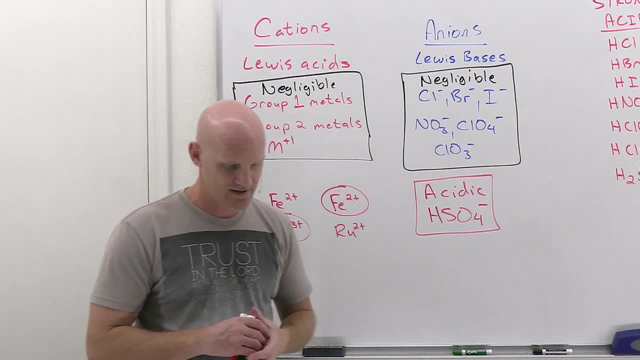 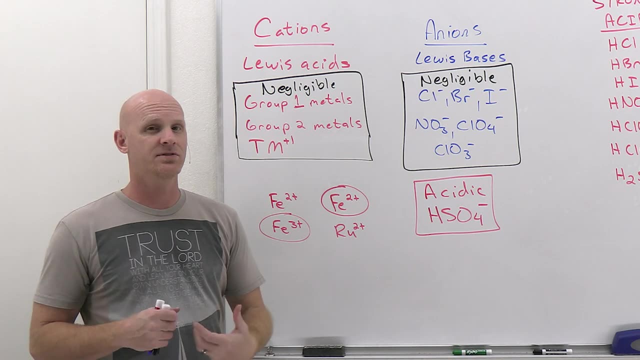 And that's just a quick aside on a couple trends there For these Lewis acids. So what you might be asked now, then, is we're going to present you with some salts and you're going to have to identify if these salts are acidic salts, basic salts. 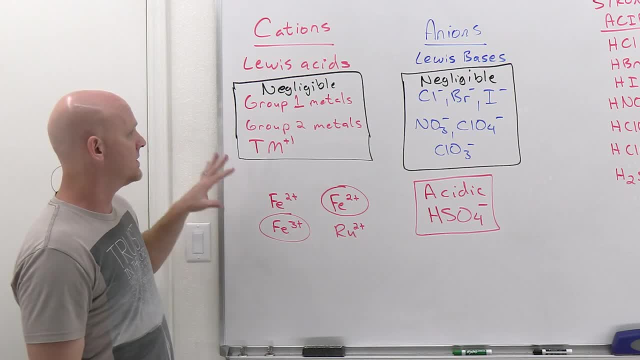 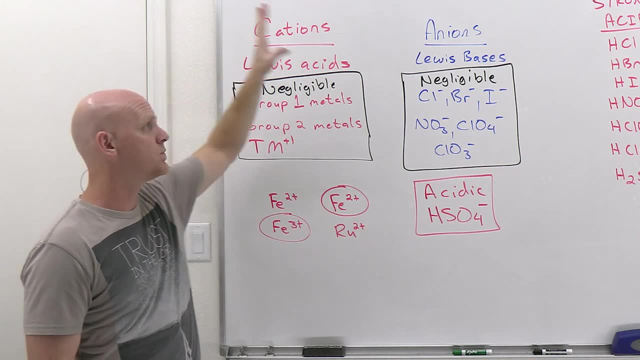 or neutral salts. And the idea is, you know, if you've got negligible cations and negligible anions, that's going to be a neutral salt, But if you've got an acidic cation with a negligible anion, that's going to be an acidic salt, But if you've got a negligible cation with, 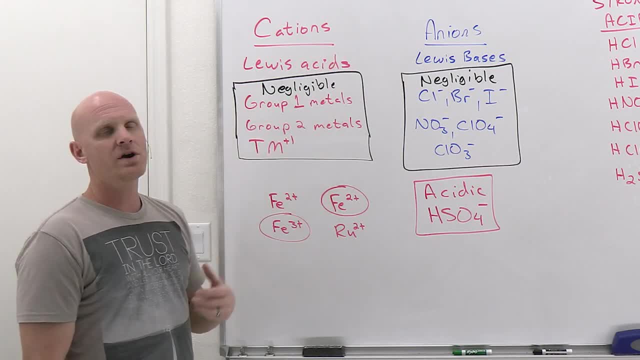 a basic anion. that's going to be a basic salt. So, and odds are, you're probably not going to have one of each. You're probably not going to have both an acidic cation and a basic anion- not the most likely scenario. The only case you might see that is if you have a hydroxide salt. 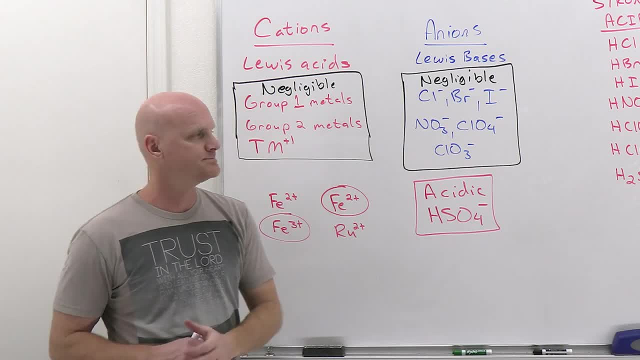 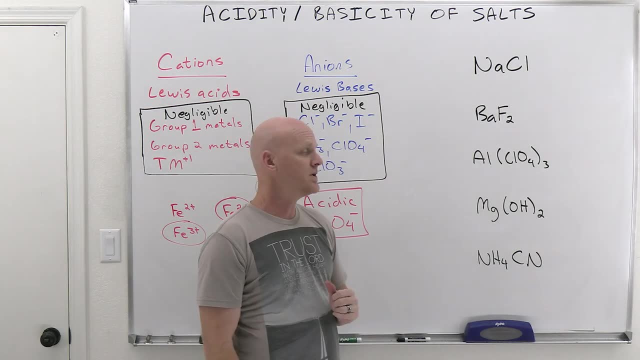 and you should just think that hydroxide salts are going to be bases, because it's hydroxide. All right, So let's take a look at a few examples. All right, So here we've got five ionic compounds. These are the ones we're going to run through, So, and when you look at these, you should realize. 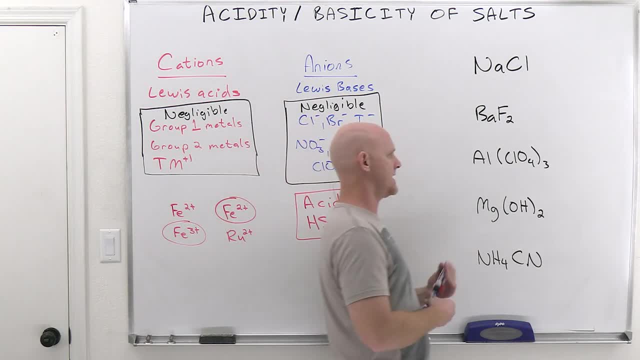 oh well, magnesium hydroxide is one of your strong bases. So, right off the bat, if you've got a strong base for one of your ionic compounds, well then that's going to be a base And, in fact, even if it wasn't. 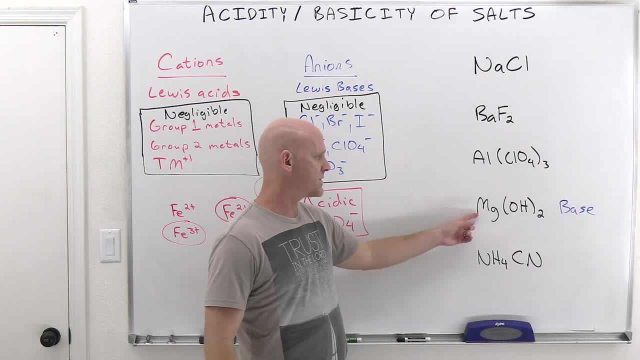 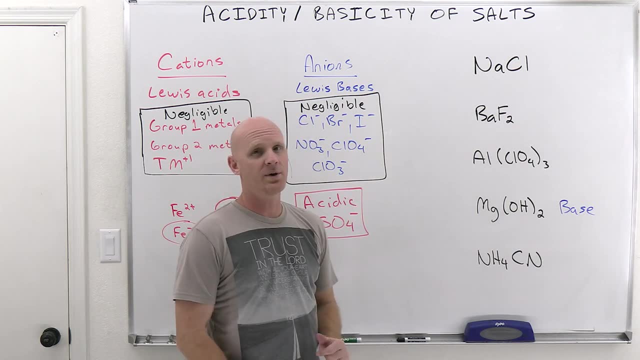 a strong base. hydroxide salts just tend to be basic, So, regardless of what the cation, they're probably going to be base. In fact, I can't think of an example, but it's not going to be the case. So the other four, though, we're going to evaluate here and we'll come back through. 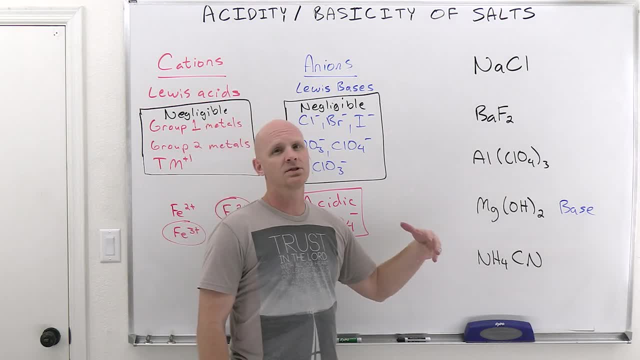 him and just verify some things. But for the other four, what you want to do is look at your cations, And oftentimes you get this in a context of a multiple choice question, where you're going to get several answer choices And rather than looking at each answer choice separately, 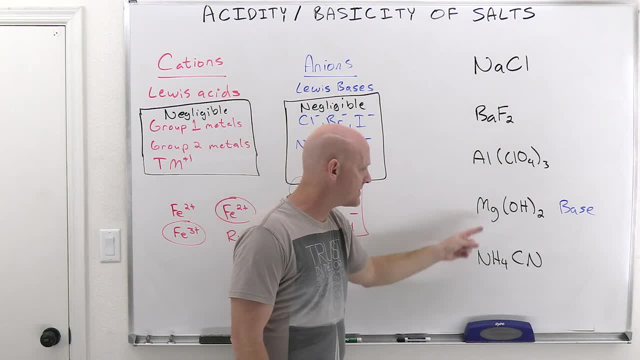 I'm just going to go through and examine all the cations at the same time. So because when I look at cations, I'm just going to go through and examine all the cations at the same time. So because when I look at cations, 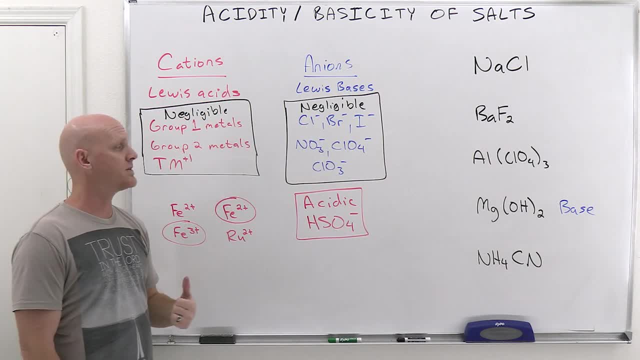 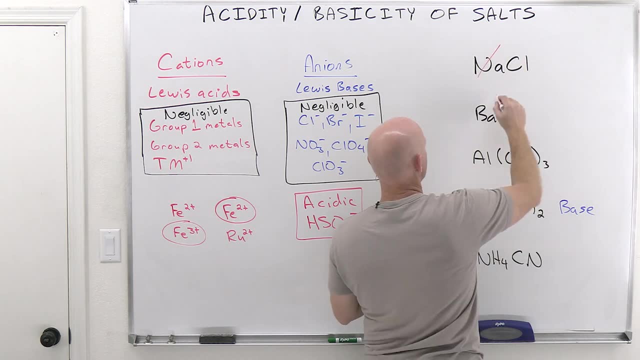 I think, oh, group one and group two, or if it's a transition metal, that's only plus one. those are the ones I'm going to eliminate. So if you look, then we can say that sodium is group one, barium is group two, magnesium is group two, but aluminum is not group one or two. 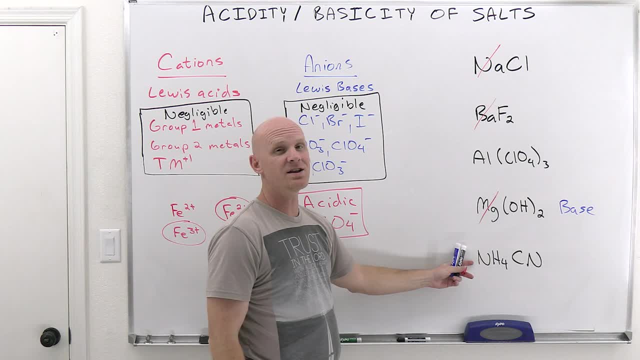 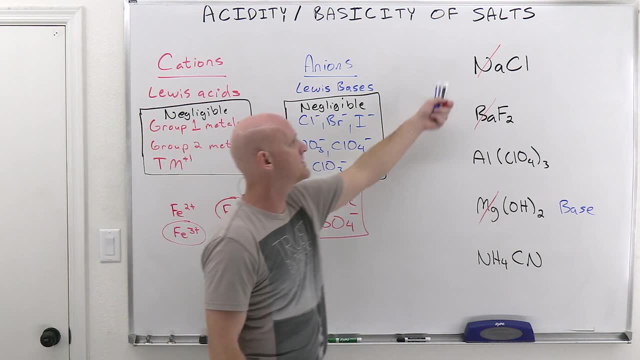 and it's got a plus three charge, so we can't ignore it. And then ammonium is not even a metal, it's a polyatomic ion, So he's definitely not in the negligible category here and is therefore an acid. Anybody that we didn't cross out as negligible is going to be an acid for a cation. 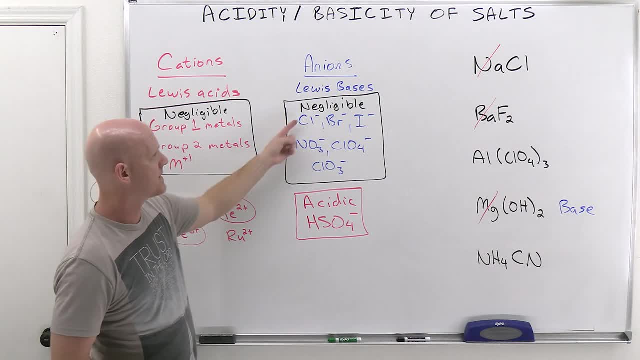 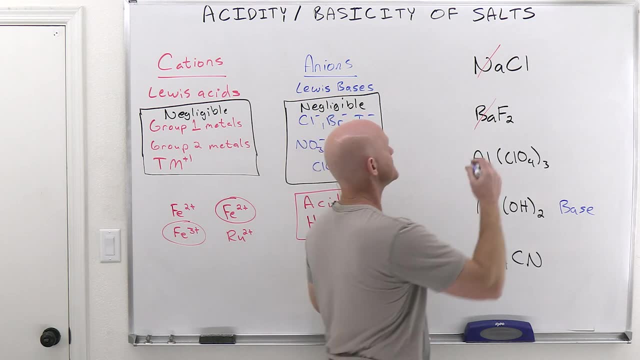 Then we'll move on to the anions and analyze it the same way. Anybody that was the conjugate acid of six out of those seven strong acids, that conjugate base is going to be negligible. HCl is a strong acid, so we can cross off chloride. HF is not a strong acid though. 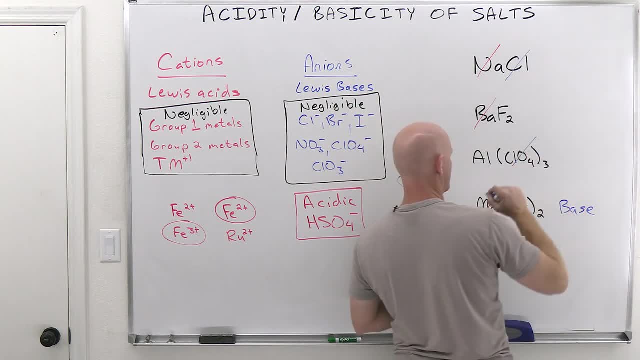 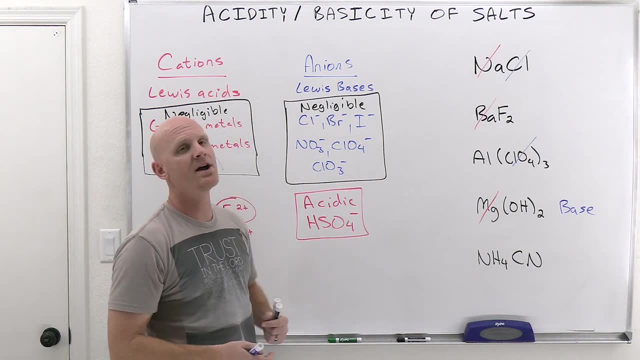 and F minus doesn't appear in the negligible list here. HCl of four is a strong acid and that's it. We crossed off a couple. That's the way it goes. So if you notice, then some people actually say: you know, split your ionic compound up and with your cations. 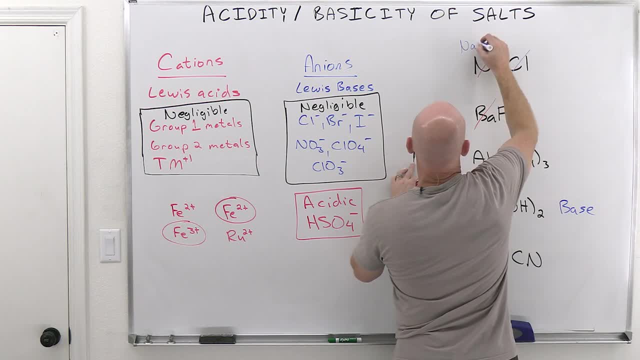 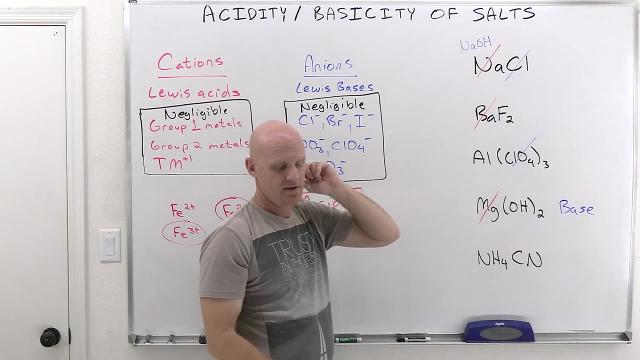 add an OH. And if what you just made is a strong base like NaOH is, then cross off your cation. So, and then on the other side they say to your anion, add the H first. And if what you write is: 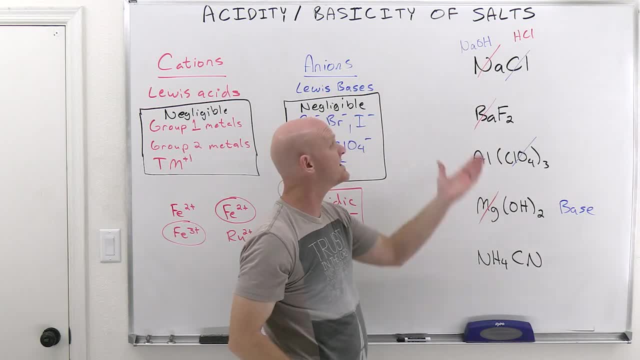 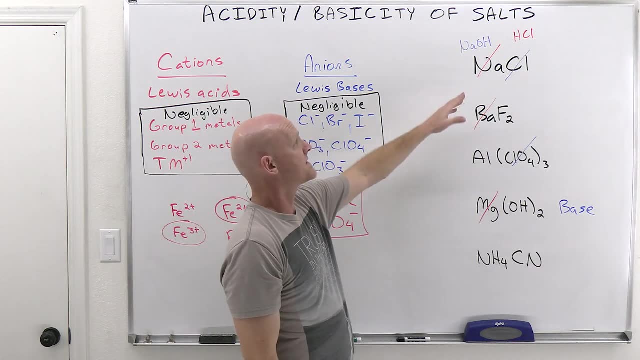 a strong acid, then cross him off. He's going to be a negligible conjugate base, And that's another way to approach this, Not personally the way I do it, but if it works for you, fantastic, All right. So the way this works now, if you've crossed off your cation, 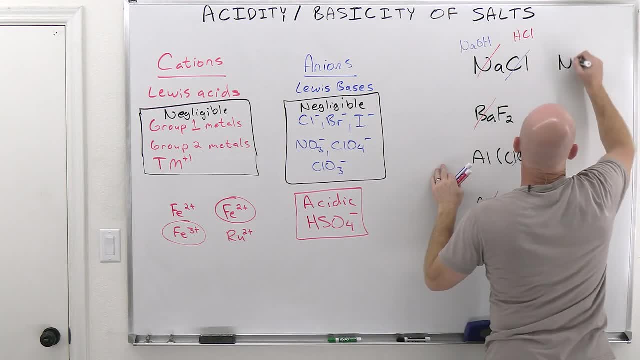 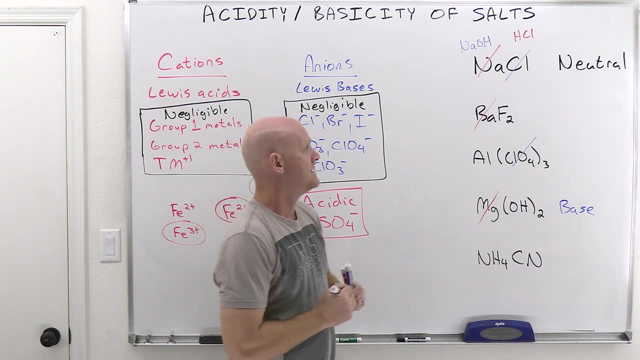 is negligible and your anion is negligible. well then, that right, there is a neutral salt. You can add it into water and the pH is going to stay right around seven. Now, if you've crossed off your cation, but you have not crossed off your anion. 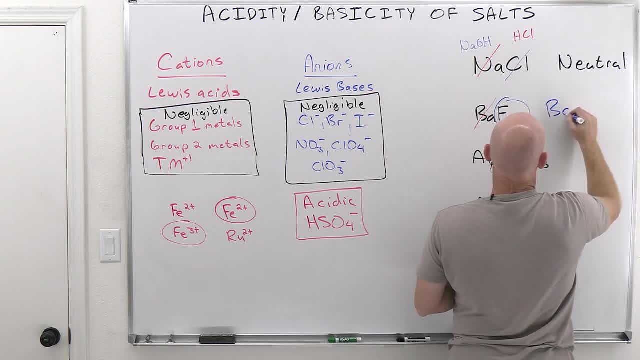 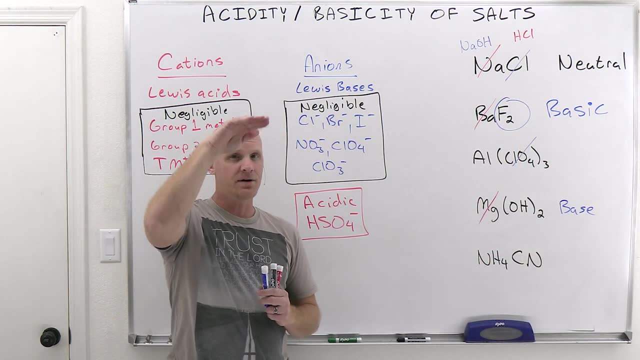 well, almost all anions are bases and this is going to be a basic salt. Cool, You stick barium, fluoride and water and the pH is going to go up above seven. All right. On the other side of the equation here we've got aluminum perchlorate. 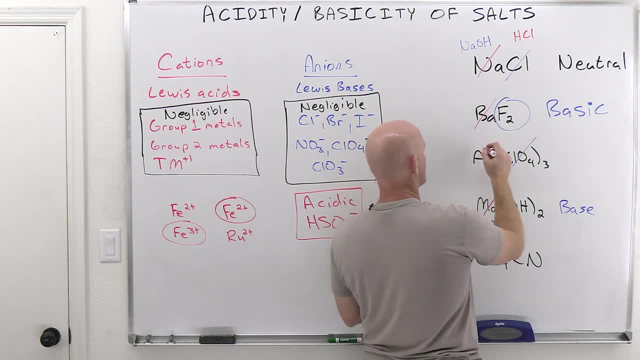 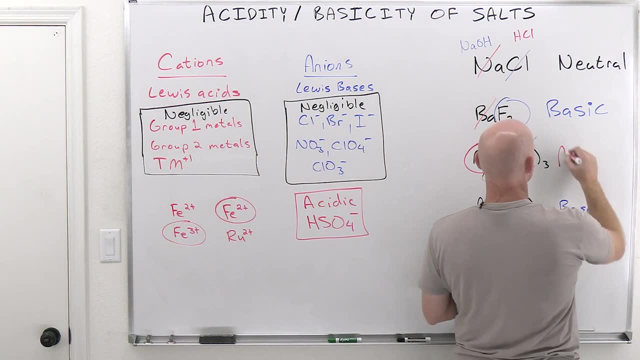 and again we've crossed off the anion, but aluminum we did not cross off and any cations you didn't cross off are acids And you put aluminum perchlorate in water and the pH is going to go below seven. It is definitely an acidic salt, As we said before with magnesium. 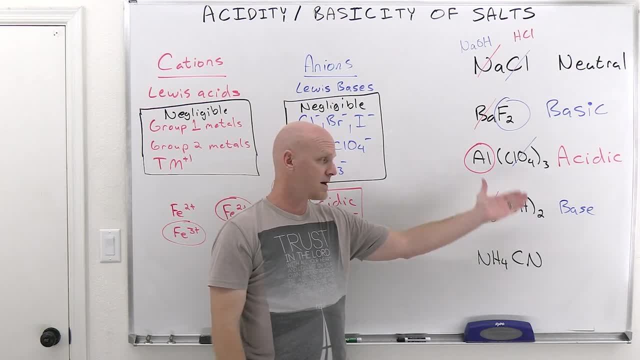 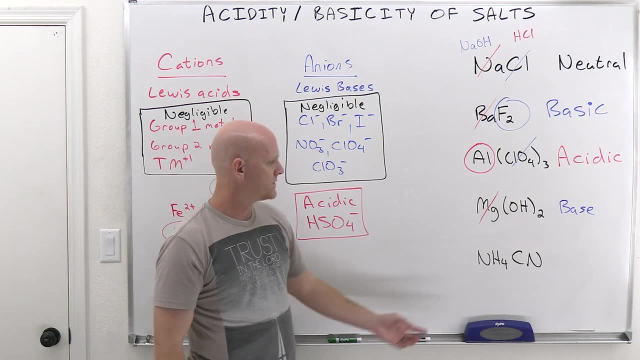 hydroxide. we crossed off the cation, but we have an anion that's a base. so obviously the base- and in this case it was a strong base, Cool. Now the last one is not fair. So with this last one we've got ammonium. We didn't cross him off, He's an acid. 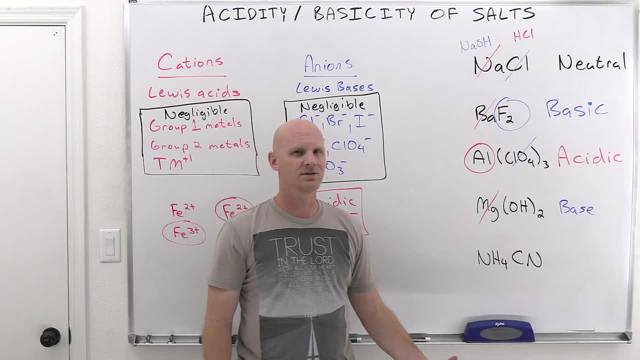 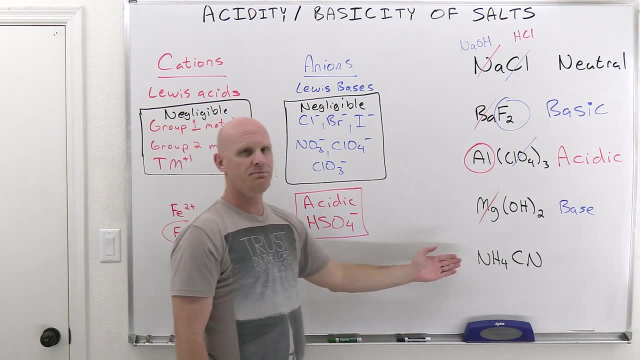 And then we've got cyanide on the other side. We didn't cross him off, so he's a base, So you didn't have a negligible for either the cation or the anion. If you recall, a second ago I said you're not going to see this and then I put it on the board. Well, I just wanted to give. 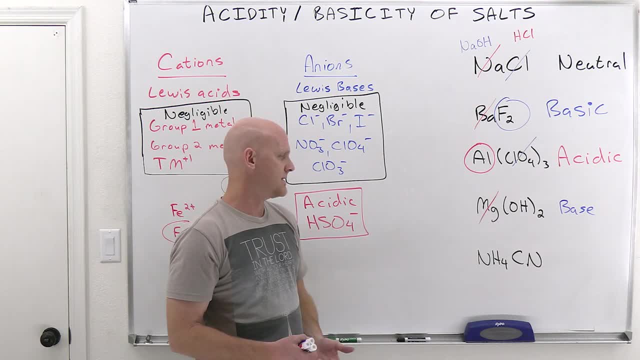 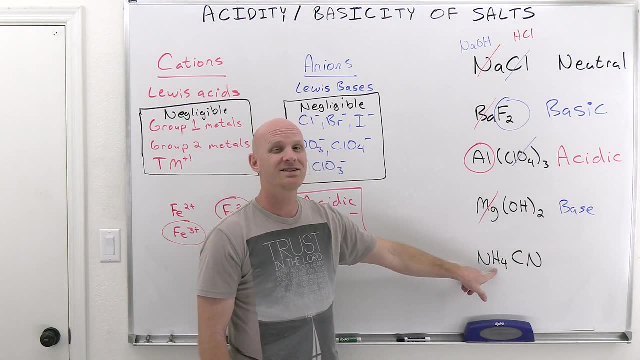 you an example of what you're probably not likely to see and you could actually answer this if you could look up some values in a table and stuff like that. And what you'd really need is you'd need the ammonium ions Ka and you'd need the cyanide ions Kb And you'd probably have to look. 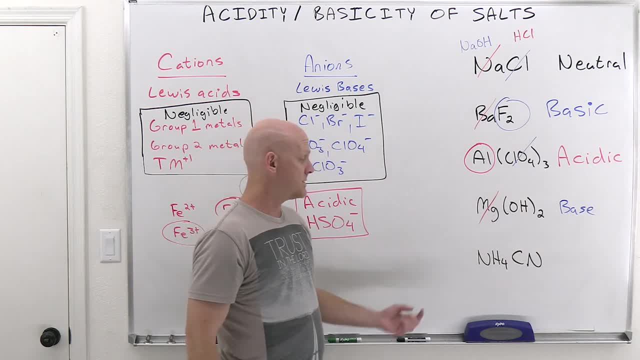 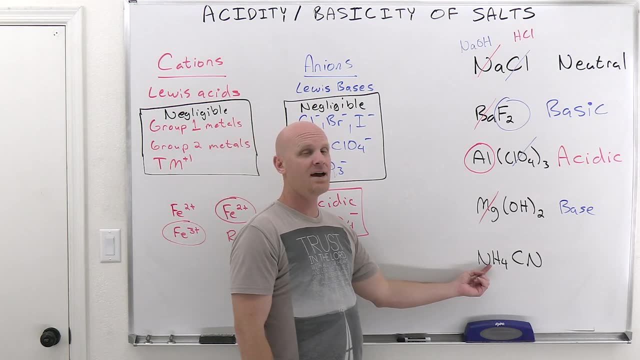 and then actually determine them, as we'll see in a little bit here. But basically, whoever's got the higher Ka or Kb, that's the one that's going to win. So if ammonium's Ka is higher than cyanide's Kb, then it's going to be an acid, But if cyanide's Kb is higher than ammonium's Ka, 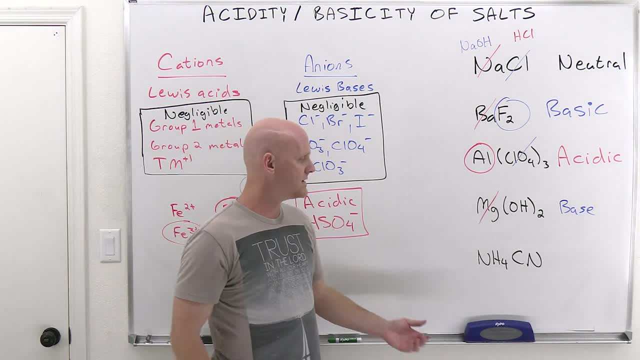 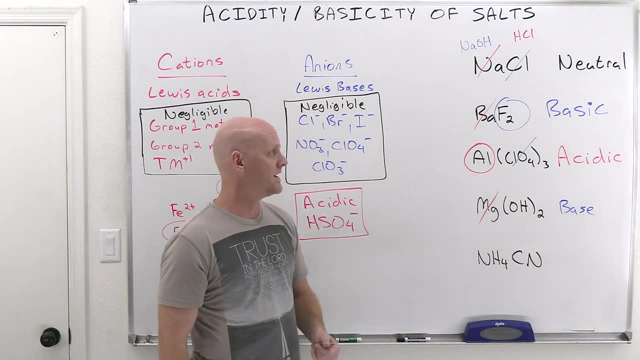 then overall it would be more basic salt. But if you don't have Ka's and Kb's, then you just can't answer this question. It's not something you're likely to encounter in that scenario, So just keep that in mind. So now we know how to identify neutral salts. a set 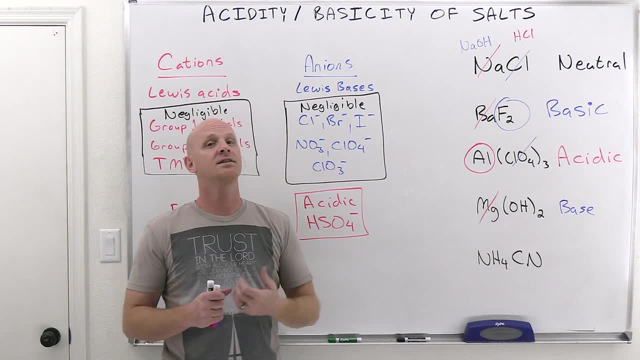 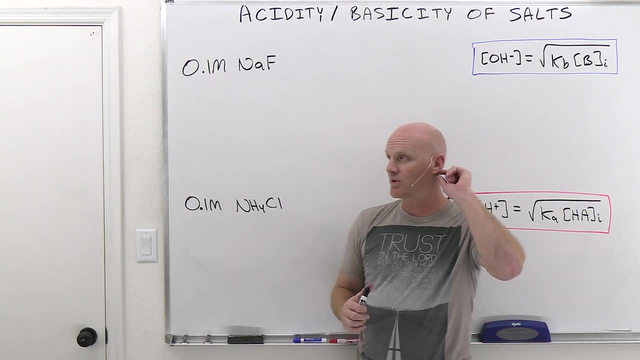 acidic salts, basic salts. So what if you're actually asked to calculate the pH of one of these salts? Let's take a gander, All right. so now we're going to calculate the pH of a couple of salt solutions. One of them is going to be 0.1 molar sodium fluoride. One of them is going to be 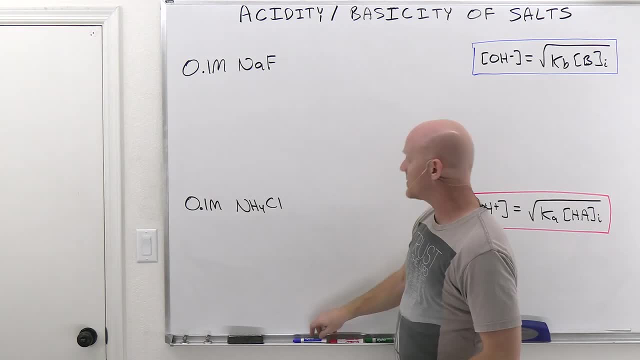 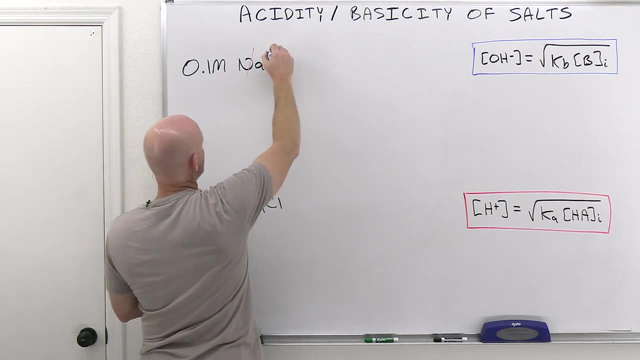 0.1 molar ammonium chloride, And if you take a look here, so sodium is a group one metal, so he's negligible. But fluoride is not the conjugate base of a strong acid. He's not negligible And so overall this is a- B. 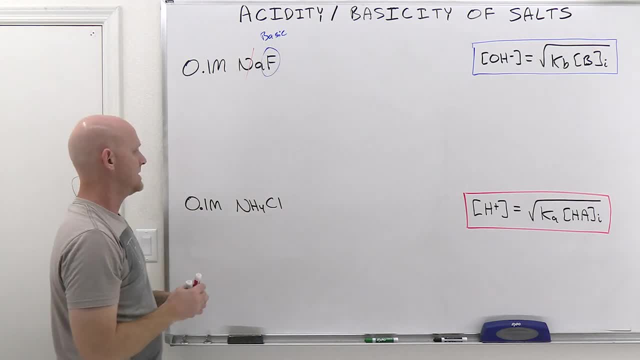 Now if we look at ammonium chloride on the other hand. so in this case chloride is the conjugate base of a strong acid, so he's negligible. But the ammonium ion is not a group one metal, It's not a group two metal, It's not a metal at all. So it's not a transition metal with a plus one. 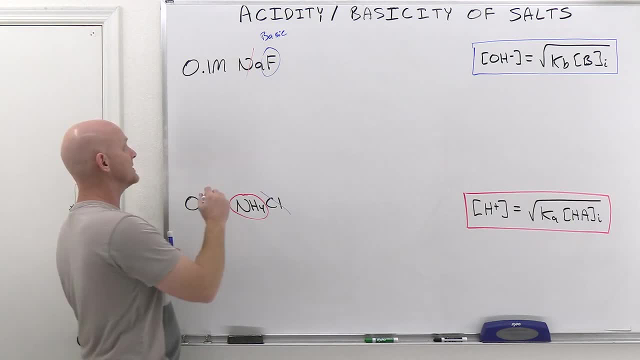 charge either. It's a polyatomic ion here, definitely a weak acid, And so, overall, this is an acidic salt and we should expect the pH to be below seven. So how would we actually go about calculating the pH here? Well, in this case, we have to ask ourselves: well, we've 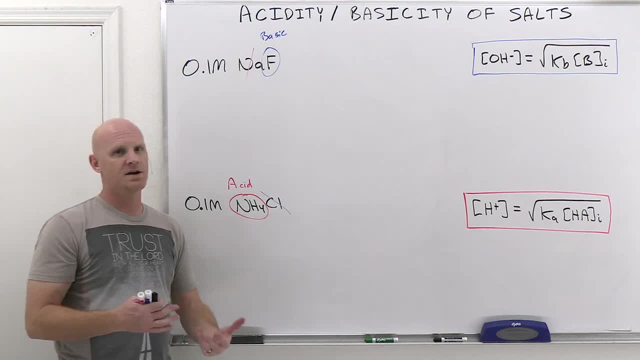 learned how to calculate the pH of strong acids and strong bases, weak acids and weak bases. Well, what do we have? Well, in this case, we've got the fluoride ion as a base. Well, the question then is: is it a strong base or a weak base? Well, it's not a strong base, because the strong bases 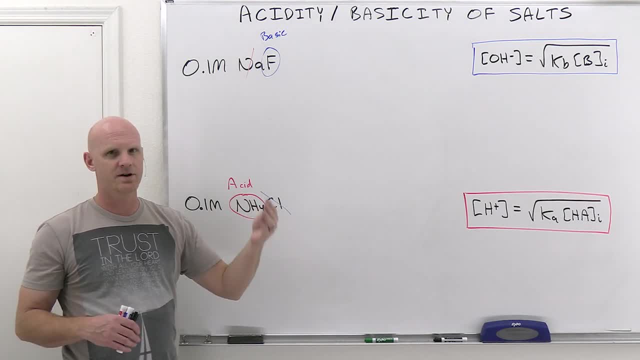 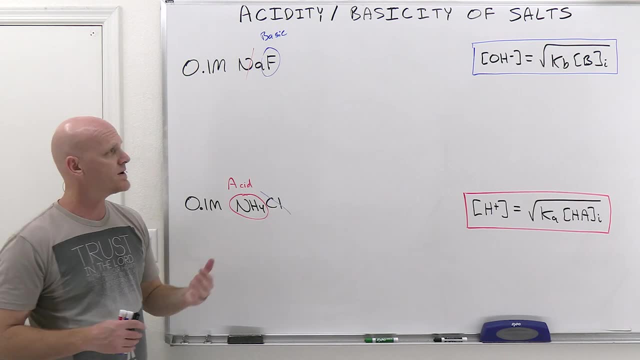 were either like lithium hydroxide, sodium hydroxide, potassium hydroxide, rubidium hydroxide, cesium hydroxide, or the group two, metal hydroxides, and he's not any of those, So he's a weak base. Well, how do you calculate the pH of a weak base? Well, we had a little. 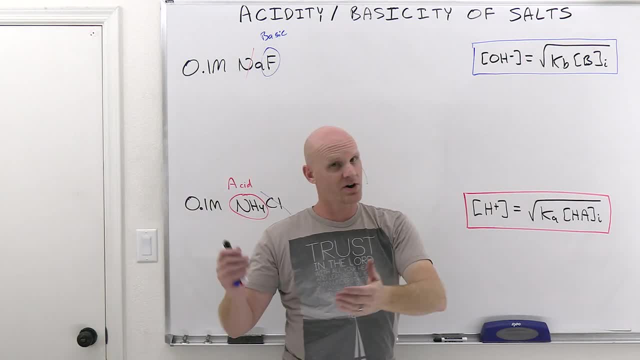 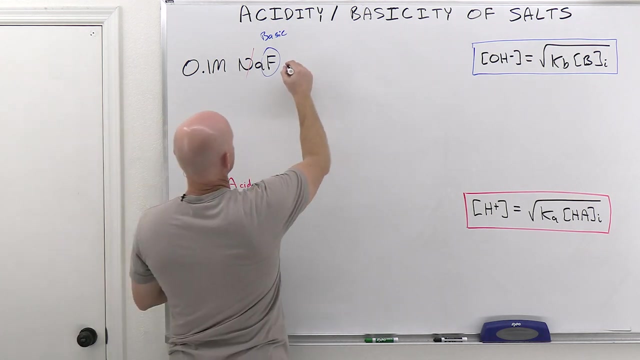 shortcut for it, right? So we technically like ice chart and Kb and stuff, but the shortcut was equals. you know, the hydroxide concentration is equal to the square root of the Kb times, the initial base concentration. So you need a Kb value. That is a problem. So what's going on here is your. 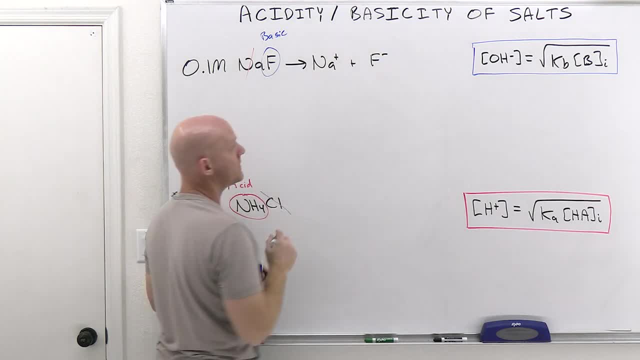 sodium fluoride is dissociating, to give sodium, and then and fluoride ions, and then your fluoride. the sodium again is not doing to do anything from that point. So, but sodium salts are completely soluble. It dissociates in ions And then that fluoride is going to further dissociate in water. 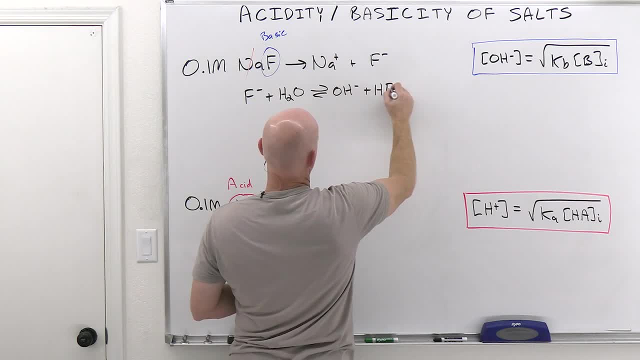 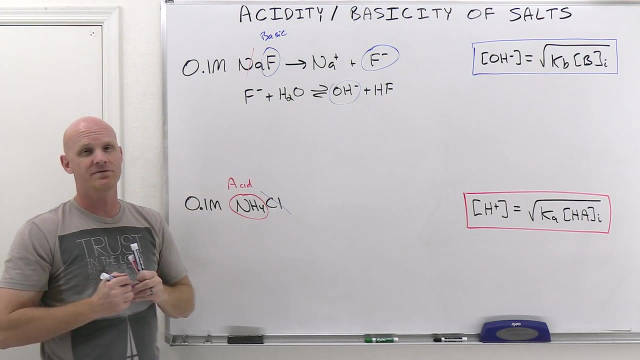 to produce hydroxide and HF. That's where your hydroxide is going to come from. So and again, the key is we said that he was a basic anion. What do bases do They dissociate in water to form hydroxide? That's where that's coming from And the shortcut we got for calculating. 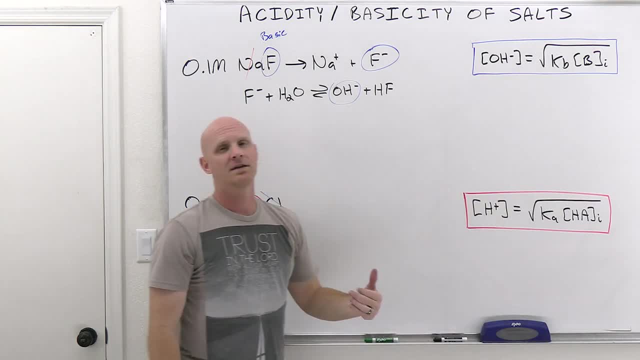 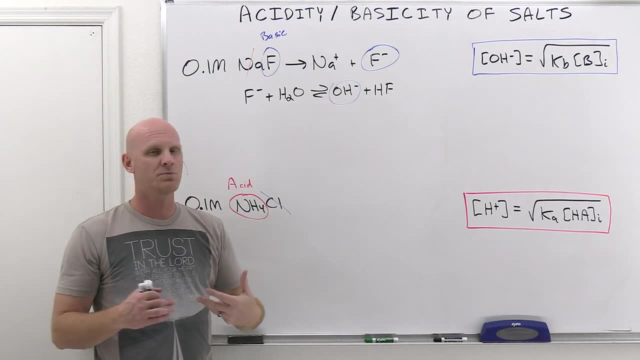 the hydroxide concentration of weak base is this guy? So we need a Kb, And so you look in the back of your textbook and you try to find a Kb value for F minus and you're not going to find it. So Kb's are most commonly reported for neutral species, neutral acids or neutral bases. 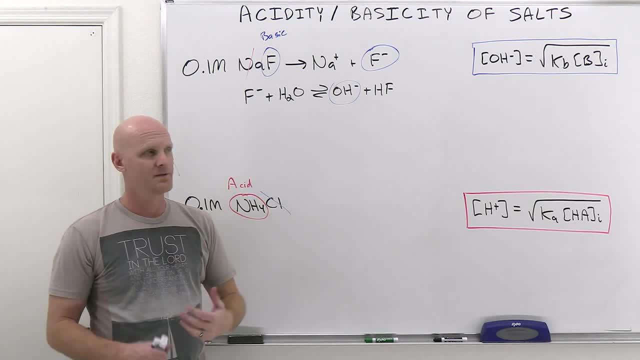 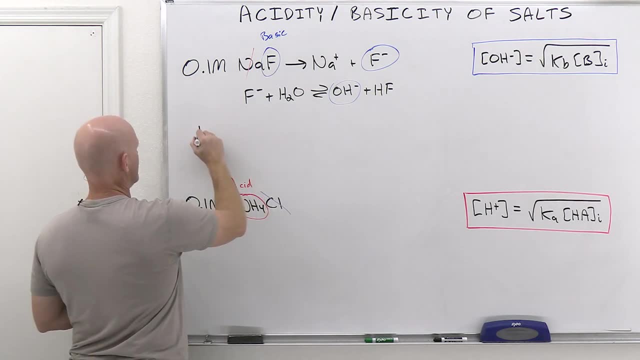 When I say neutral, I don't mean pH seven, I mean no charge, not ions, And so, in this case, you're not going to find one for HF, And that kind of sucks. What you are going to find, though, is you're going to find a Ka value for HF, given just. 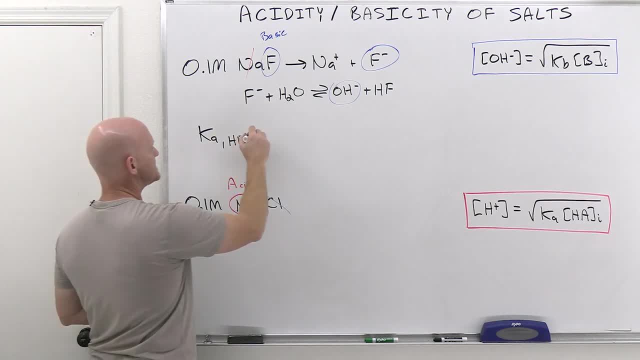 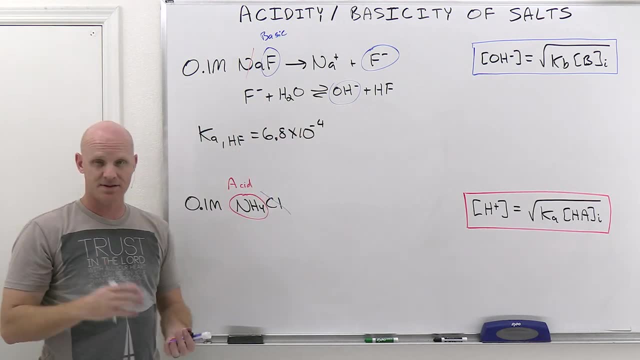 like I've provided it in this question, And so the Ka for HF is 6.8 times 10 to the negative four. So HF is a neutral species. You could totally look up his Ka in the back of your textbook and it would say something similar to this value. 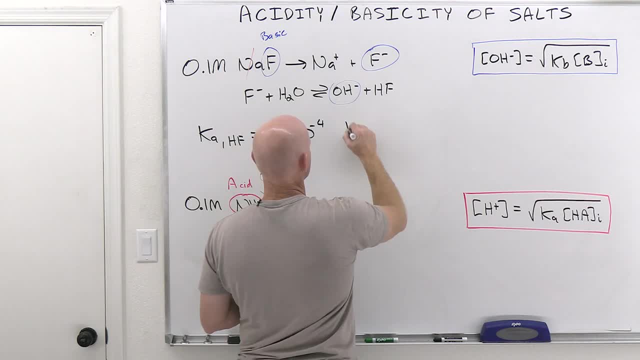 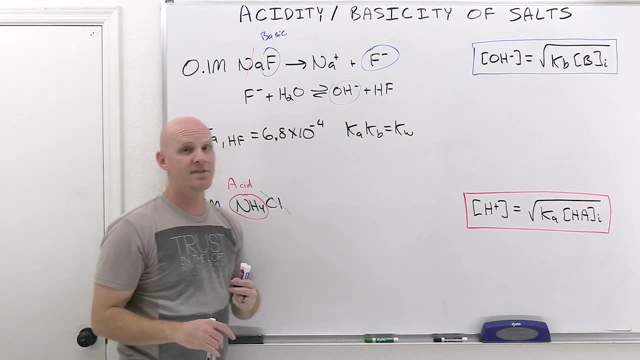 So what you're supposed to know from here is something we determined in the last lesson: that Ka times Kb equals Kw for a conjugate acid-conjugate base pair, And that's what we've got here. HF is the conjugate acid, F- is the conjugate base, And so here we need to know Kb. 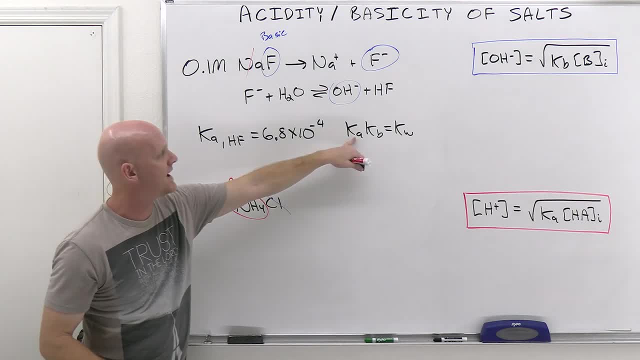 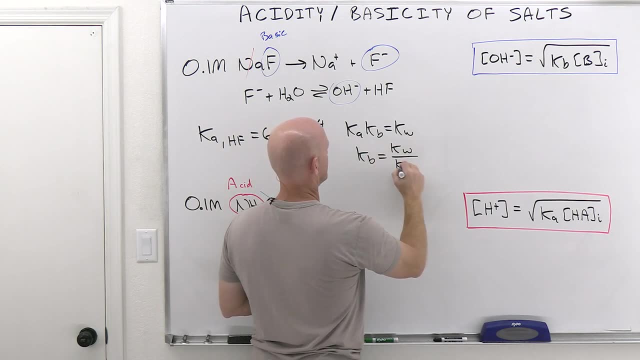 for F- but it's not going to be found in a table, most likely. So we've got to get the Ka for HF instead and really rearrange this, and Kb is simply going to equal Kw over Ka, and that's ultimately what I'm going. 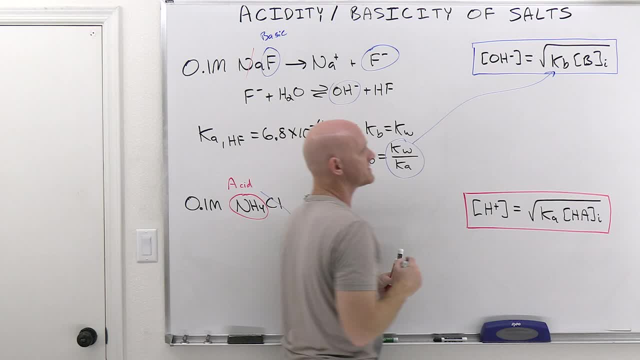 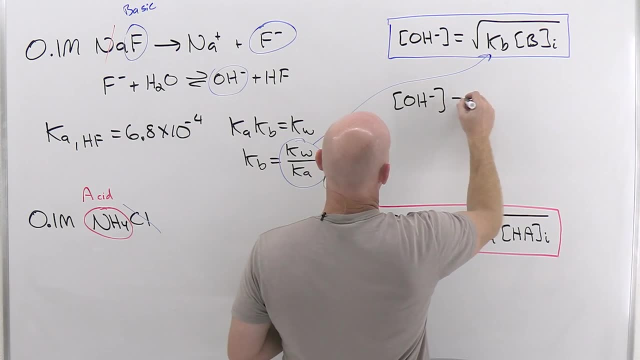 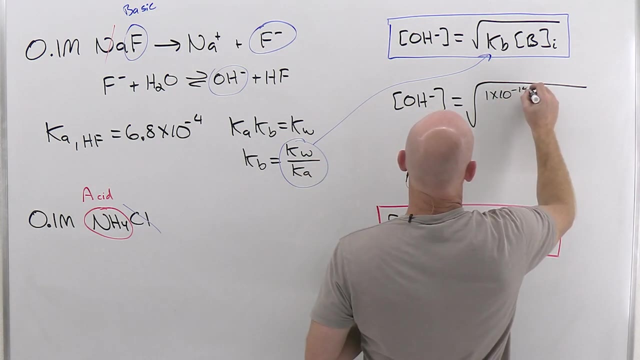 to substitute in to that expression right there for Kb. All right, so from here let's just plug in and chug in with our shortcut. So we've got hydroxide equals the square root and again Kb is going to be Kw over Ka. so that's going to be 1 times 10 to the negative 14, all over. 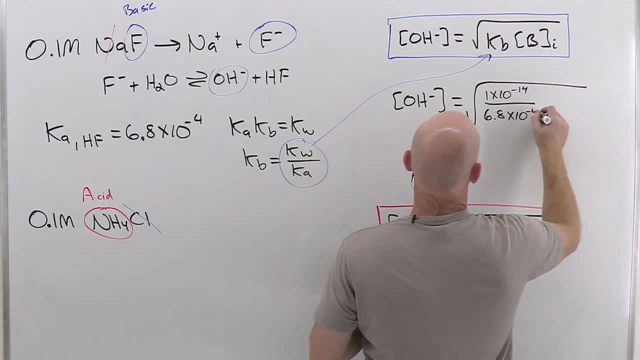 the 6.8 times 10 to the negative 4,. whether you want to calculate it first and substitute it in or just put the formula in, that's fine either way, and then we've got a 0.1 molar concentration. 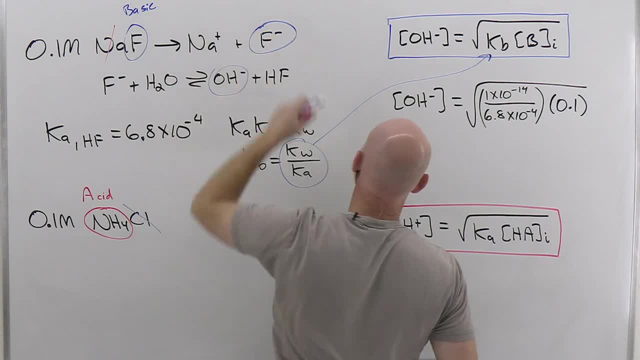 because 0.1 molar sodium fluoride- 1 to 1 ratio here should give 0.1 molar fluoride. If for some reason we had a coefficient of 2 here, well then this would be 0.2 molar. 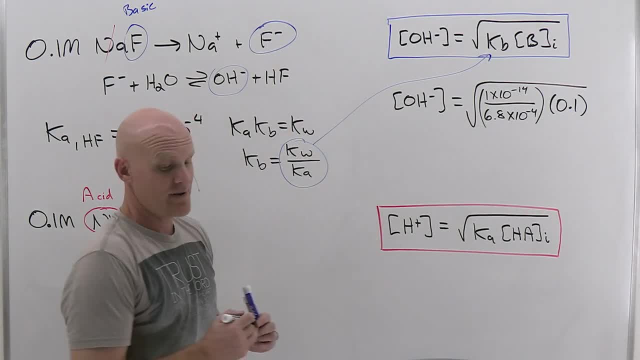 instead. but in this case it is 0.1 molar and from here it's plug and chug to get that hydroxide concentration. Let's take 1,, 2,, 3,, 4,, 5,, 6,, 7,, 8,, 9,, 10, and 10.. 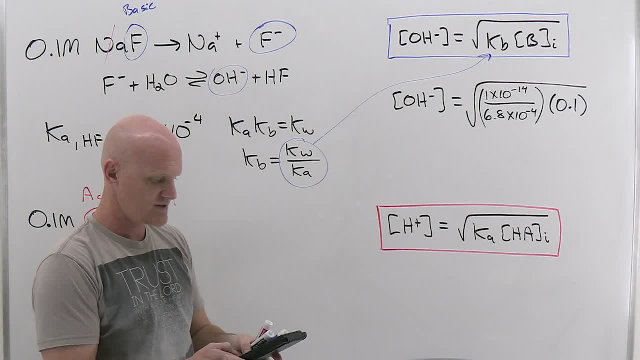 Times helps when you turn your calculator on. so 1 times 10 to the negative 14.. Need my hand Divided by 6.8 times 10 to the negative, 4 times 0.1, and that's going to be. 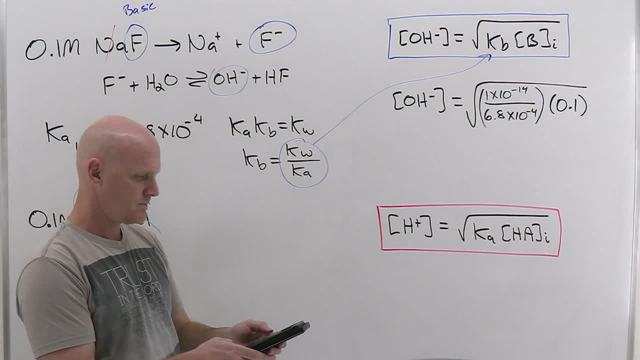 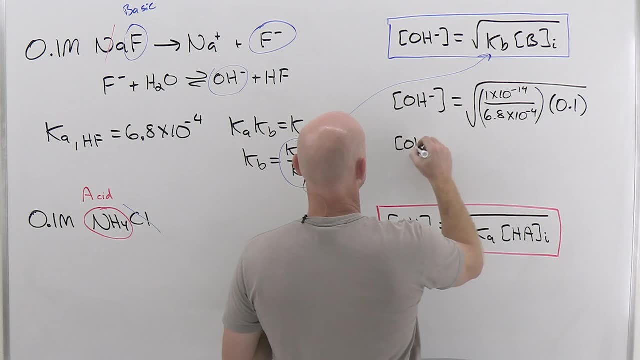 1.47 times 10 to the negative 12.. I'm going to take the square root of that and get 1.2 times 10 to the negative 6. Molar, And then we'll take the negative log of the hydroxide to get the pOH, so the negative. 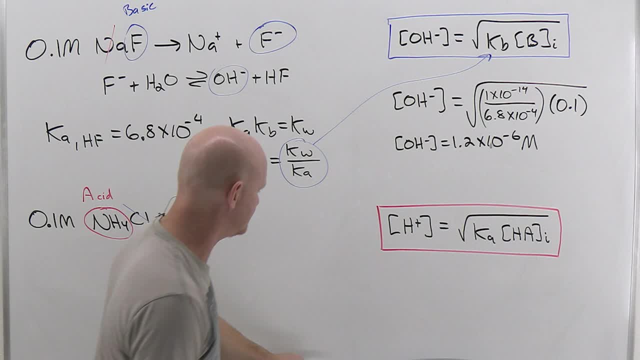 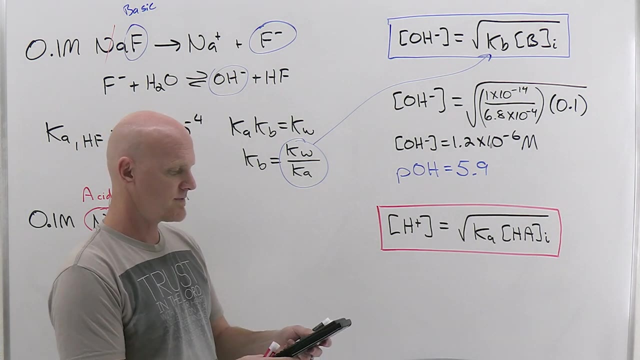 log of this number comes out to 5.9.. And if we subtract from 14 in a number like this, I just highly recommend you use your calculator 14 minus that last answer, for whatever reason. subtracting from 14 with: 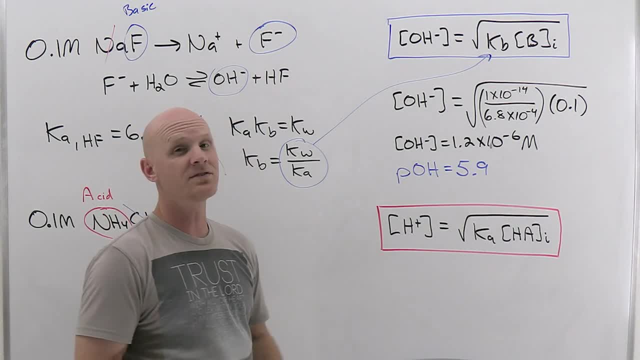 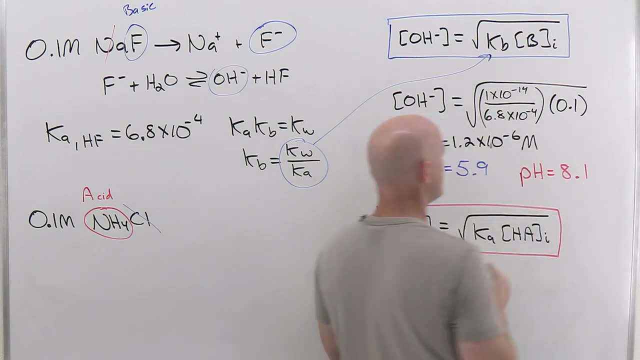 numbers and decimals is a pain in the butt. We're going to get 8.1.. A lot of students would have done this. Come out with 9.1, so I'm saying, to use your calculator, Cool, and that is your ultimate answer. There's your pH, So most salts are going to typically. 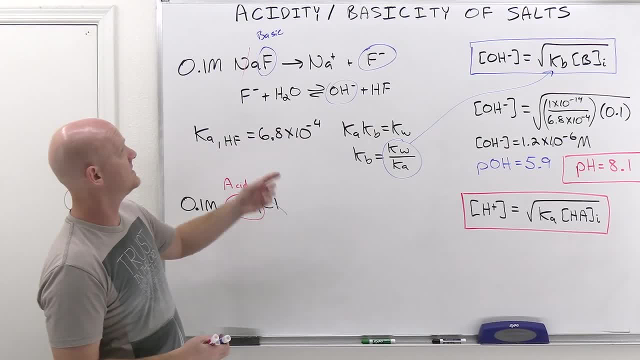 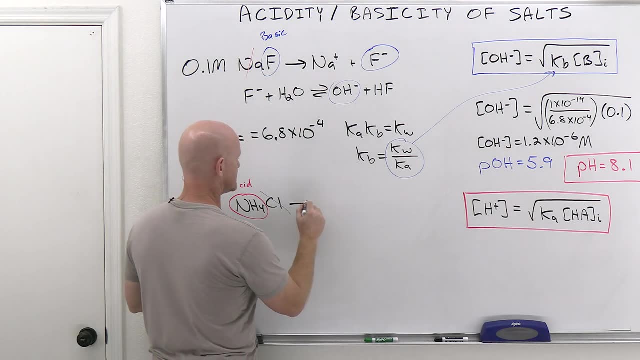 end up just being either a weak acid or a weak base, depending on. if it's the anion, then it's a weak base or, in this case, it's going to be the cation. So ammonium chloride is completely soluble in water to a very, very significant extent, and you're going to get 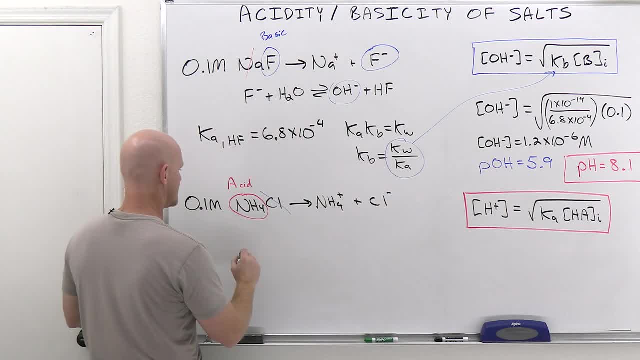 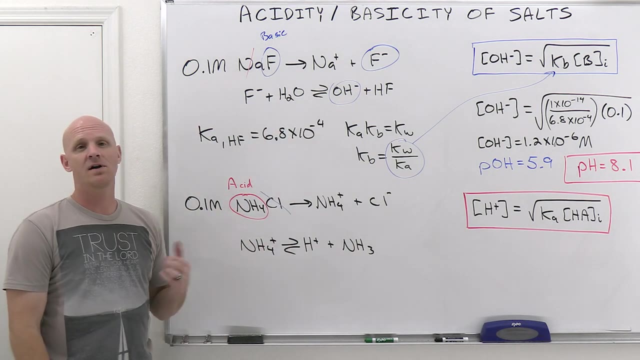 ammonium ions and chloride ions, and it's the ammonium That is a weak acid, so it's going to dissociate, to give H plus an ammonia, And once again we have an issue. though Ammonium ions have a positive charge, They're cations. 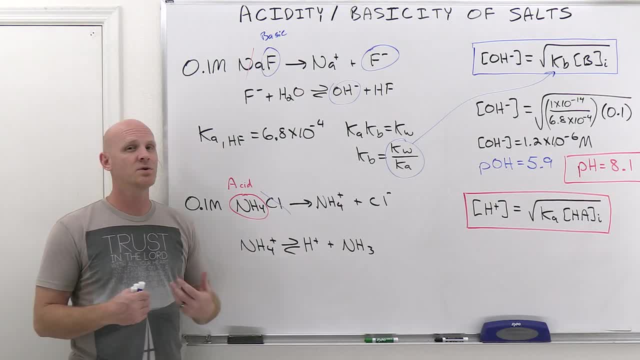 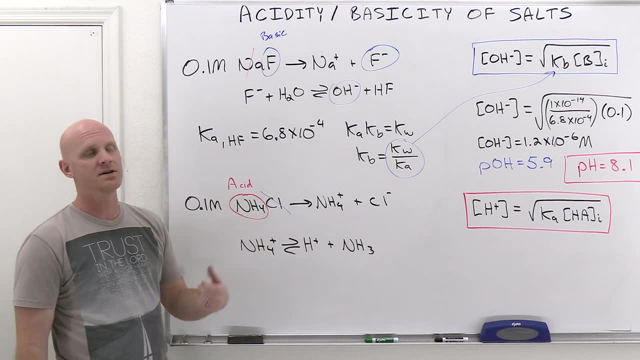 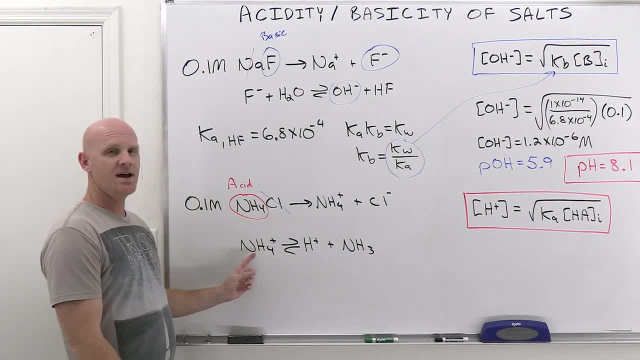 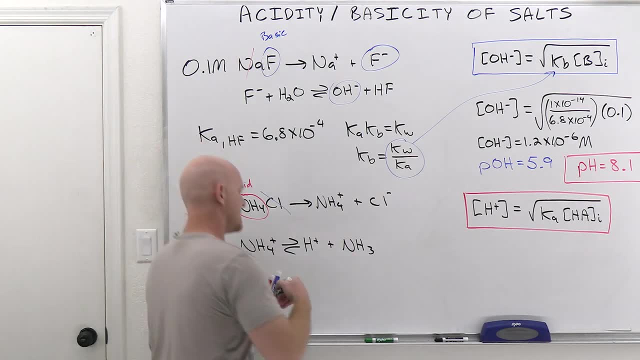 And it's in this question as well. So the key is: we're not going to find a Ka for him directly. We'll have to calculate it using the Kb for ammonia instead. And so in this case, instead of solving for Kb, we're solving for Ka. So Ka is going to equal Kw over Kb, And that's. 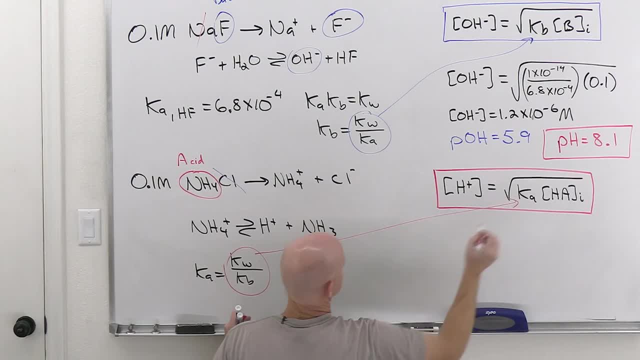 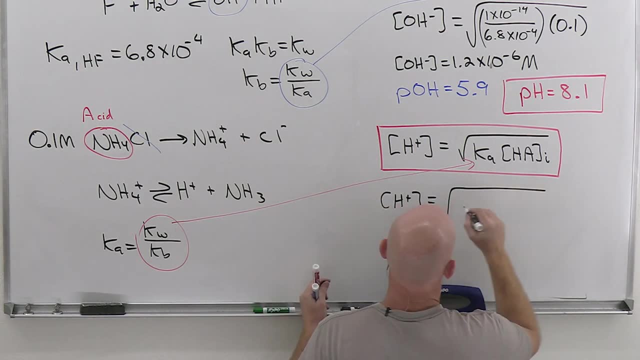 what I'm going to substitute in into our shortcut here. And so in this case our H plus concentration is equal to the Kb. And so in this case, our H plus concentration is equal to the Kb square root of 1 times 10. to the negative 14,- all over 1.75 times 10 to the negative 5 times 0.1. 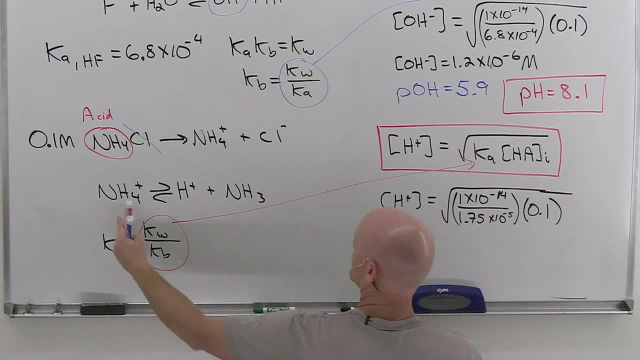 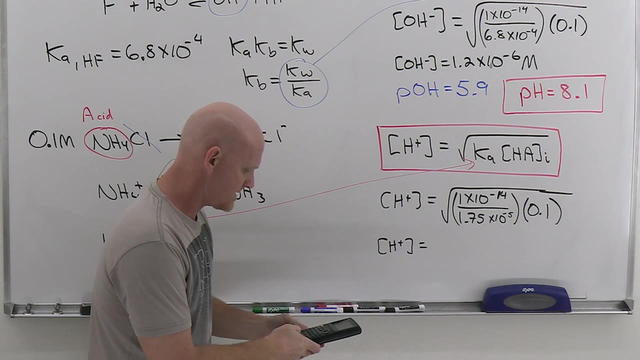 molar for our acid concentration. So because we get one ammonium from one ammonium chloride And from here it's going to be plug and chug to get our H plus and then we'll take the negative log to get the pH Pull out that calculator again. All right, so 1 times 10 to the negative. 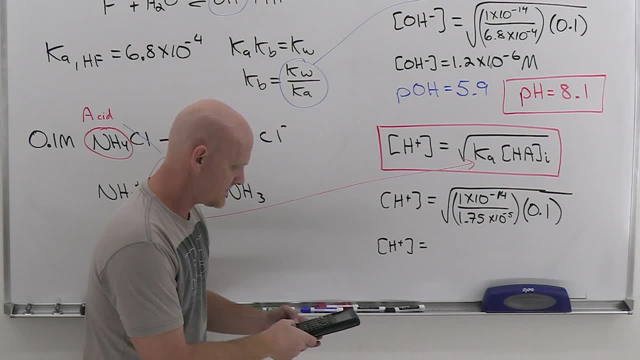 14 divided by 1.75 times 10 to the negative, 5 times 0.1 gets me 5.7 times 10 to the minus 11.. I'll take the square root of that and get 7.6 times 10 to the negative 6.. 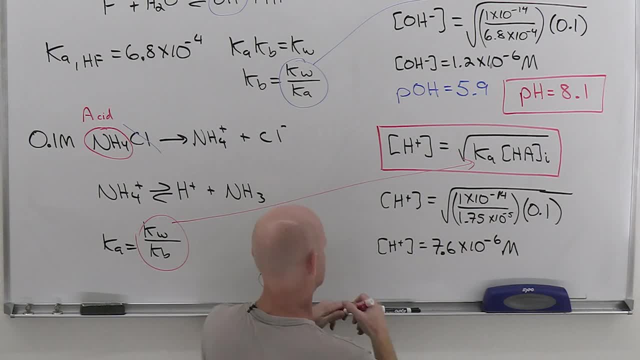 Again, we'll take the negative log of this to get the pH. So negative log of my last answer gets me 5.1.. And voila. So one thing to note. I've kind of worked these out, I've tried to make it look. 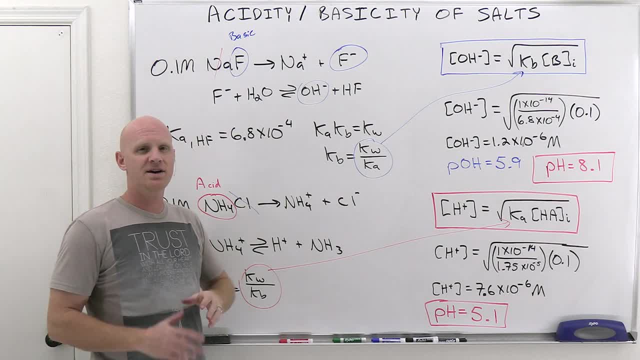 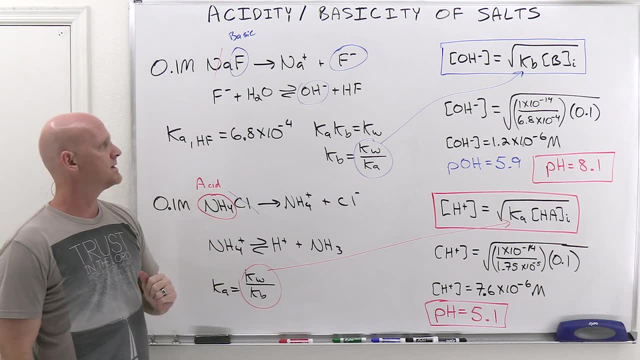 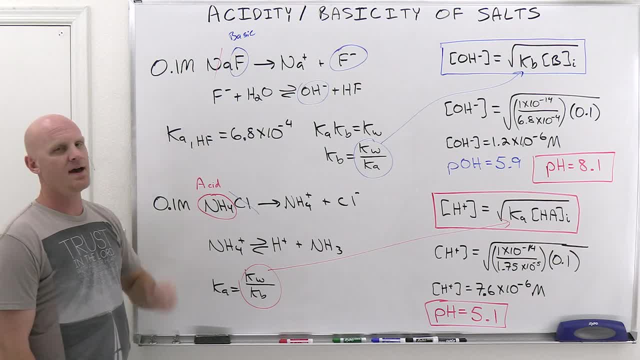 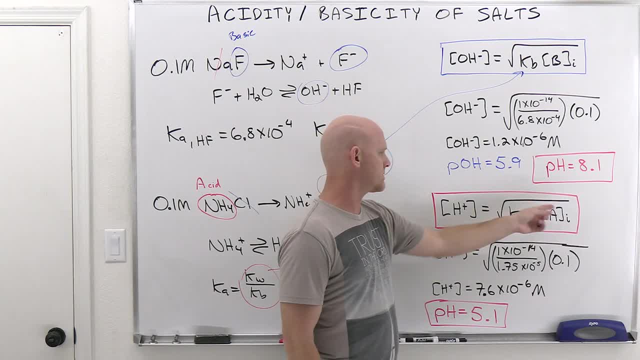 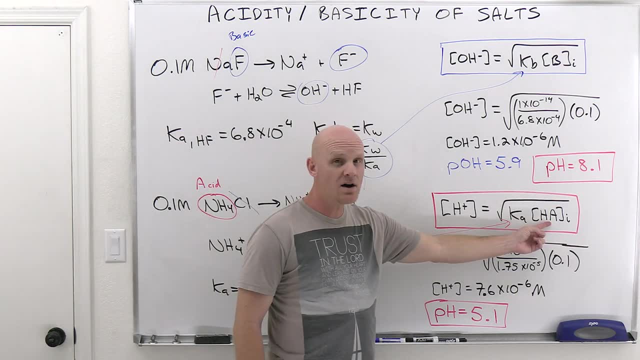 Oh, whenever I got a Ka and a concentration, I multiply them together and take the square root and I get the H+ And then I'll take the negative log and get the pH. The problem is that's assuming you have the concentration of that actual acid. 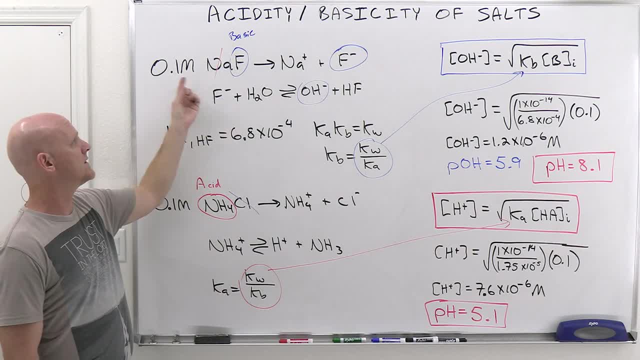 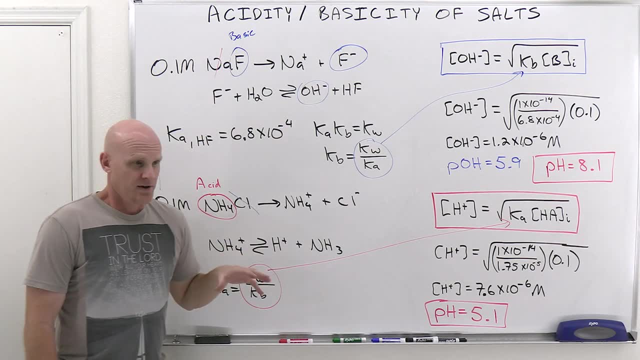 Well, I've got the Ka of HF given to you in this first example, but we don't have an HF solution. We have a sodium fluoride solution, We have a solution of the conjugate base, And so you know. there's only a handful of calculations. we have to know how to do so far. 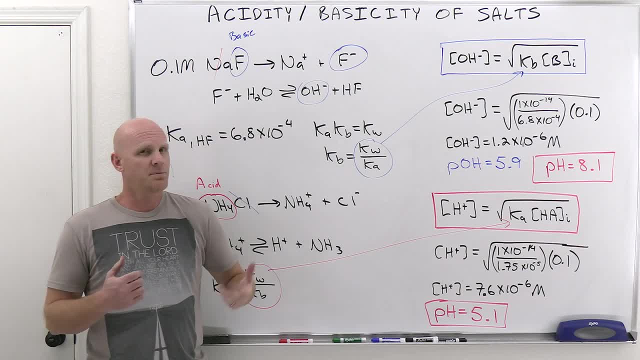 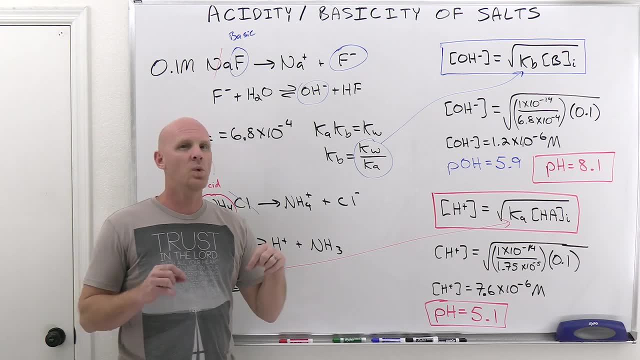 Strong acid- strong base- weak acid- weak base. So we'll add a couple more in the next chapter, but that's it for this chapter. Four different calculations that you might be on the hook for. The problem is is you've got to figure out which one you actually have. 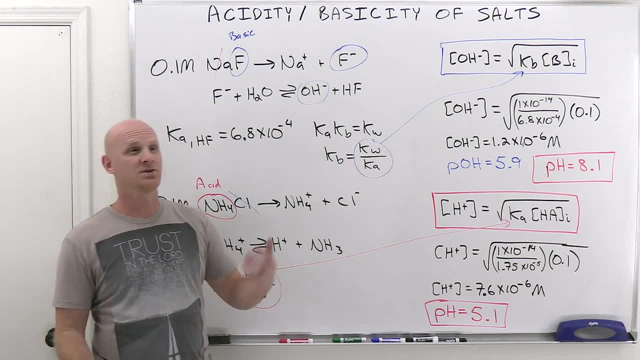 You have to be able to recognize: do you have a strong acid, Do you have a strong base, Do you have a weak acid, Do you have a weak base? And if you're given a salt, then you have to figure out which one of those that turns into after it dissociates. 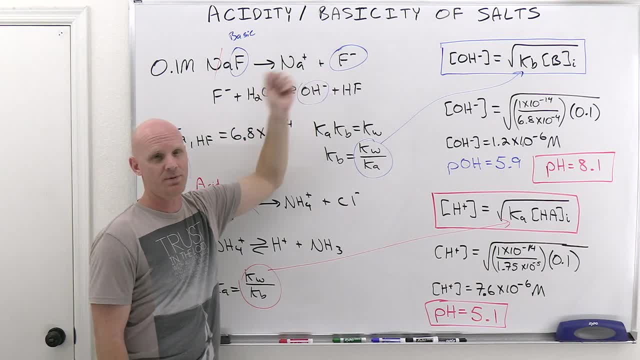 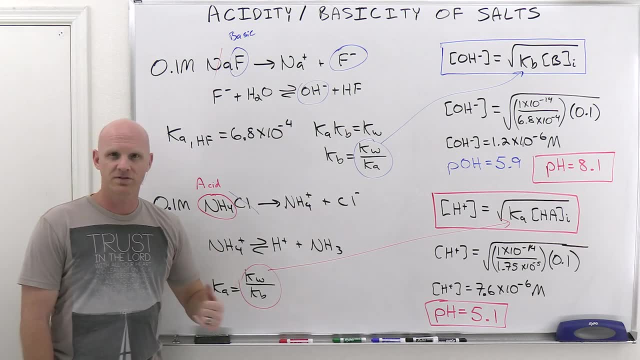 And again, in this first example, the cation was negligible, It was the anion that was a weak base. In the second example, it was the anion that was negligible, It was the cation that was a weak acid. And the moment you say, oh, I've got a weak base, there's your shortcut. 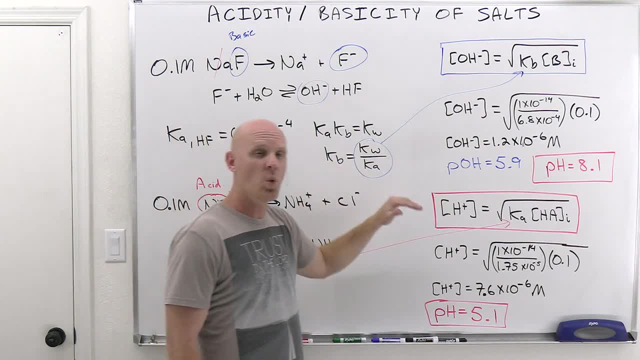 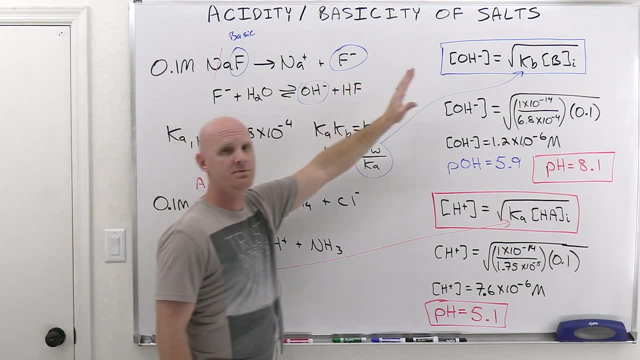 The moment you say you've got a weak acid, there's your shortcut And you have to know what to do and then look at what you've been given to figure out how you get there. So in this first example you were given a Ka, but you should have, before you, even evaluated that said. 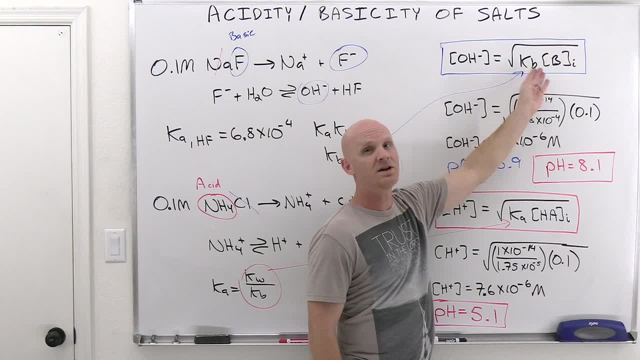 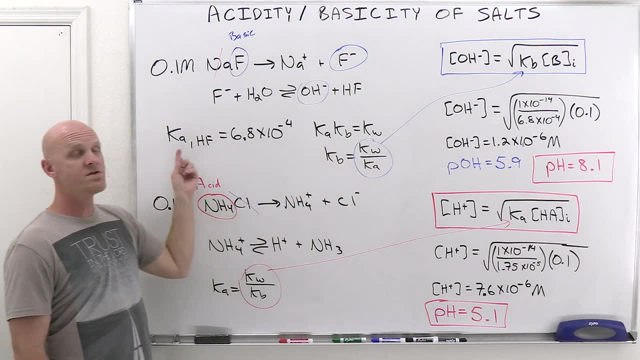 oh, this salt's a weak base For a weak base. this is my formula. I need a Kb value. Well, they didn't give you a Kb value, So you need to take and solve for Kb- Kb as equal to Kw- over the Ka of the conjugate acid they gave you. 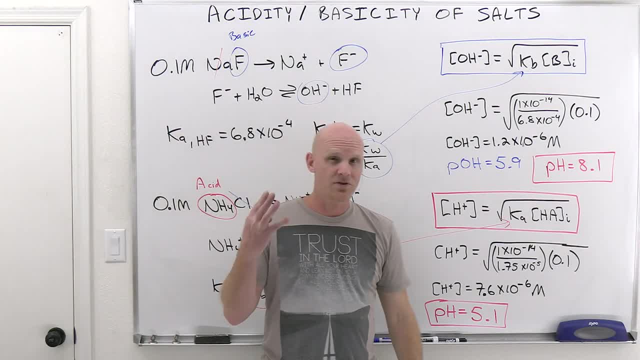 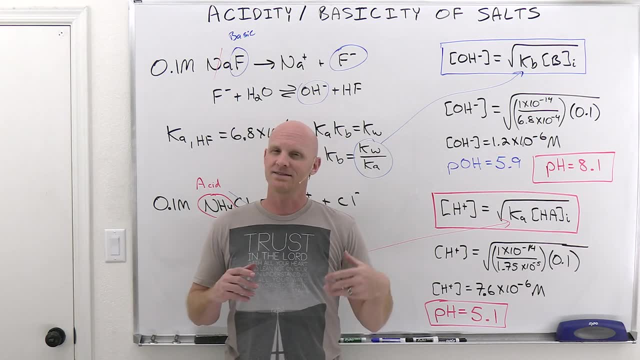 So that's kind of the methods And again, there's only so far four different types of pH calculations in this chapter, or at least four different solutions- Strong acid, strong base, Weak acid, weak base. But identifying which you have and then having it real methodical, 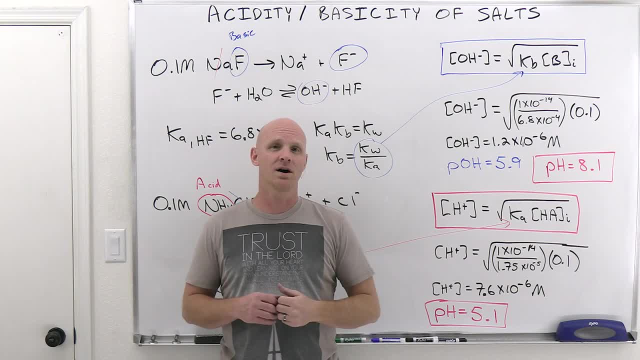 what process you're going to use to solve for that pH. that's the rub, And it's going to get more challenging because in the next chapter we're going to introduce buffers and then titrations, which are going to be even more pH calculations. 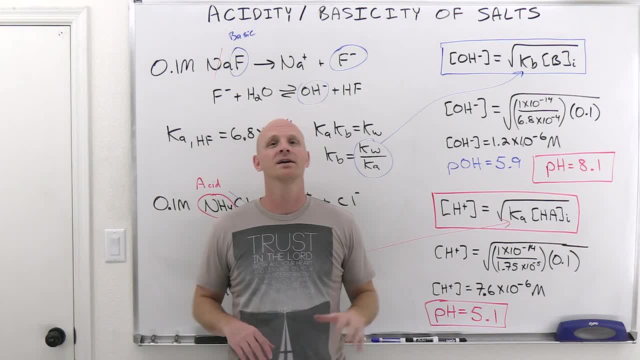 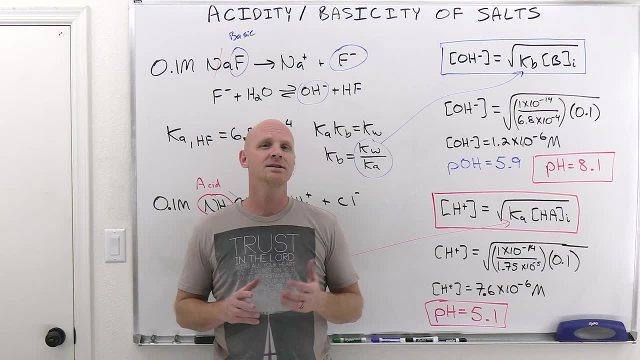 And the water's going to get pretty muddy, So you want to get this down really really good before we get into the next chapter. Now, if you found this lesson helpful, thumbs up button is the best way you can support the channel. 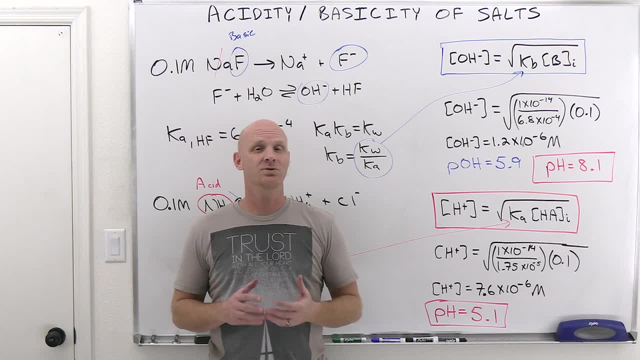 Let YouTube know that they need to share this lesson with other students. And if you're looking for acid and base practice, pH calculation practice or general chemistry practice in general, check out my general chemistry master course: Over 1,200 practice questions. final exam. rapid reviews: practice final exams. 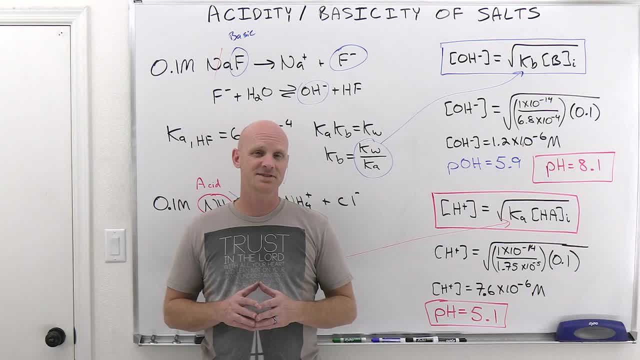 Free trial is available. I'll leave a link in the description. Happy studying.